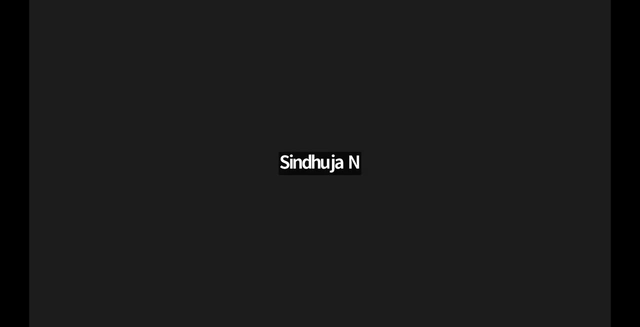 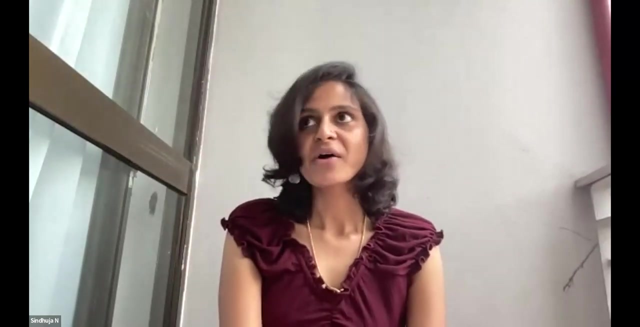 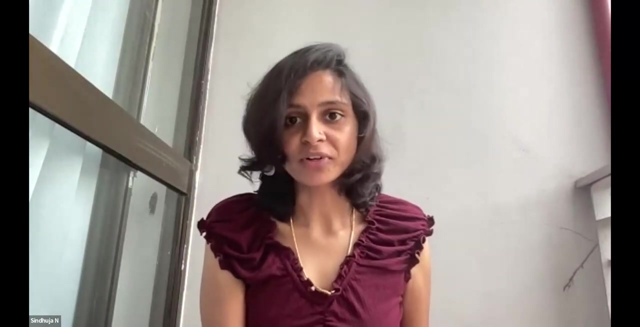 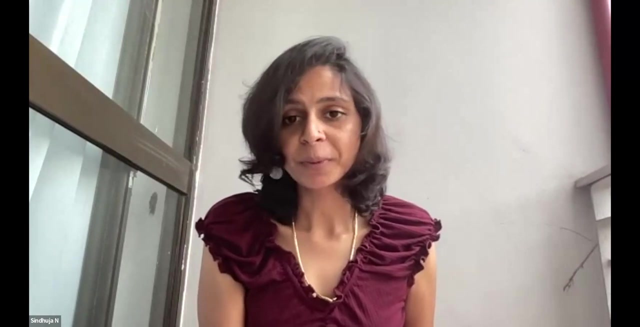 Hello everyone, good morning, good afternoon, good evening, wherever you are. And here I am with another one wonderful video of SDLC. so Software Development Lifecycle. And thank you so much, Sunan, once again, for this opportunity. Guys, this video may be a little bit longer, but trust me and trust. 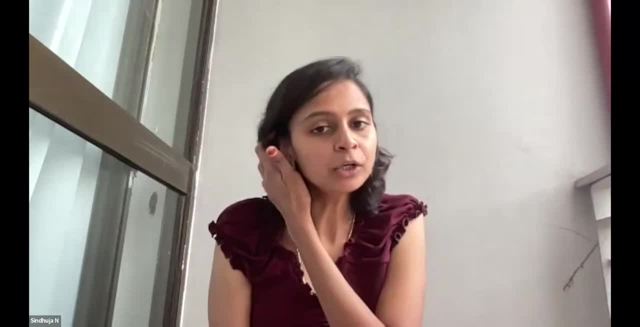 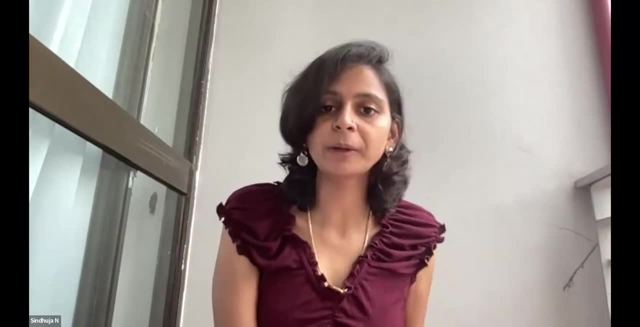 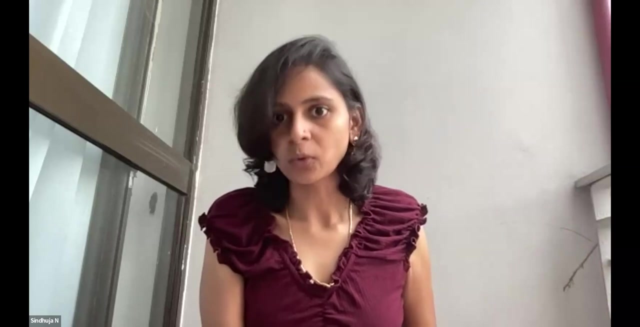 Carious Talk. it will give you complete picture, end-to-end picture, how the software development lifecycle works in the industry. This video will be very helpful for people who are switching into software industry or who are already working in software industry also. Why? Because we are all. 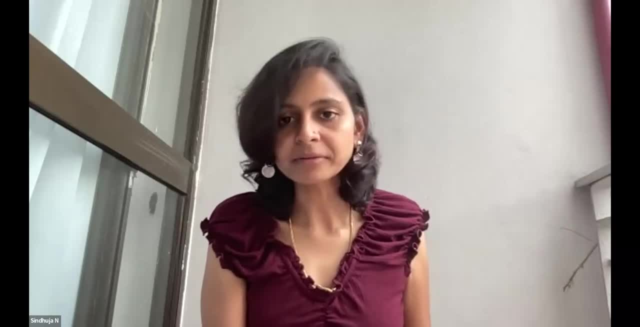 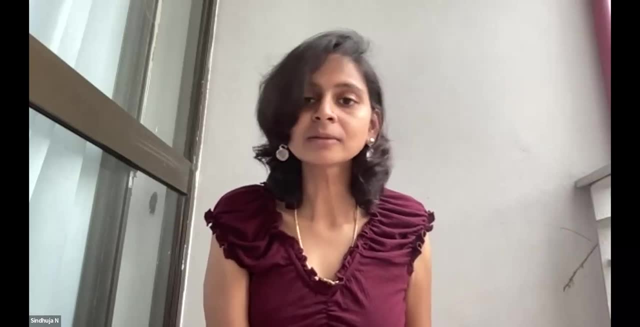 working. we must have gone through so many processes. you may have some 15 years of experience or 10 years of experience, or even, in fact, more than that, But we don't know many things which we, unknowingly, we must have done, so many things We don't know. this is what we are doing. 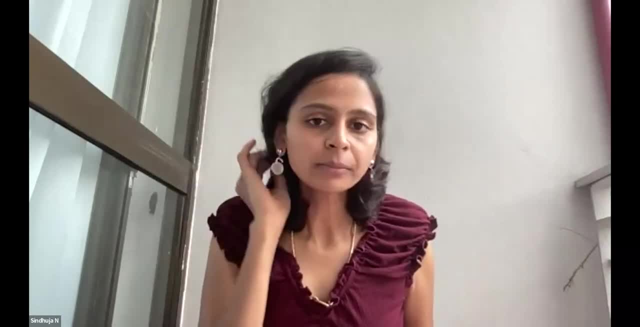 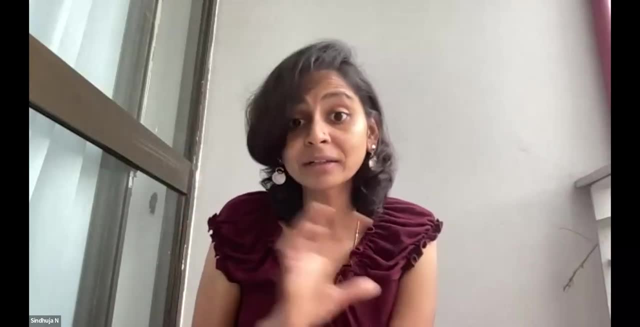 So those areas I'm going to cover today- Of course I'm not going to go in deep of each and everything because I'm cautious of time, But still you will get the better clarity and better understanding what every phase of software development lifecycle is going through, how it. 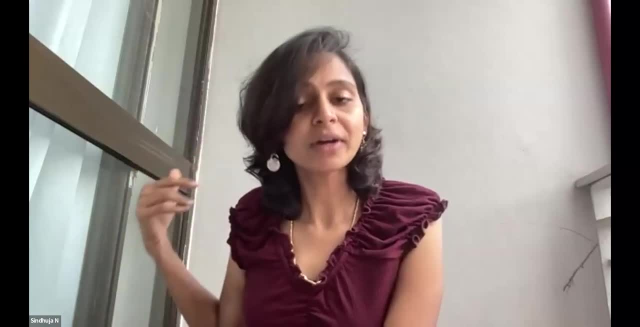 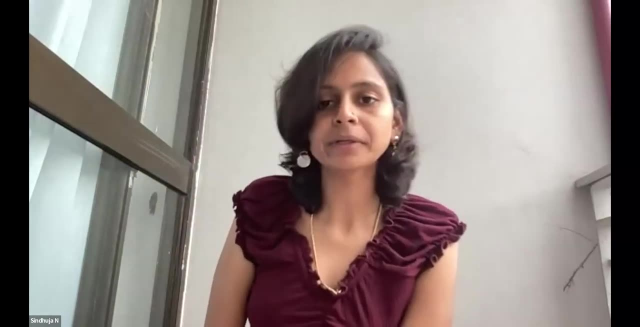 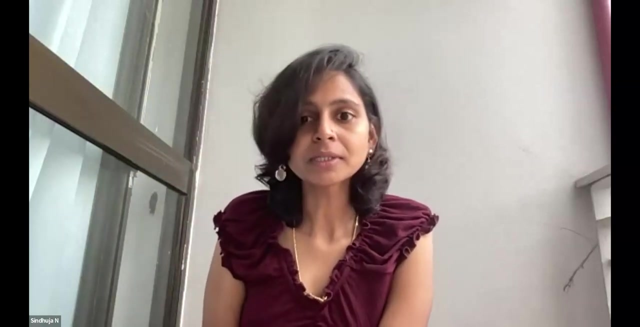 is emerges in the market And what is the final step and what are all the steps being involved. So it will be very helpful for people who are working as a developer or tester or project manager, or even a fresher or business analyst or scrum master, agile coach, because this is something basic. 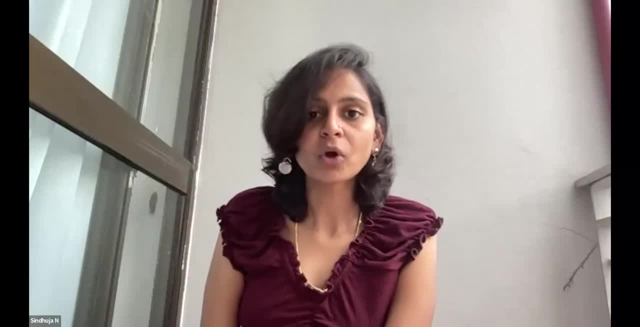 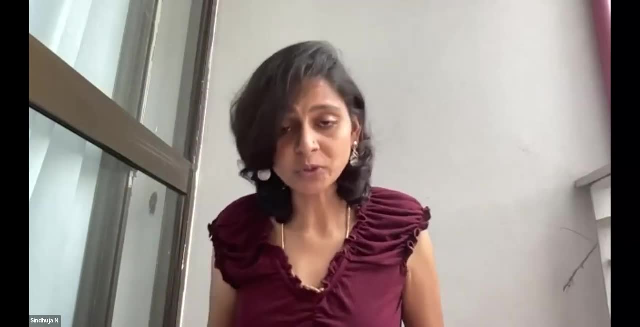 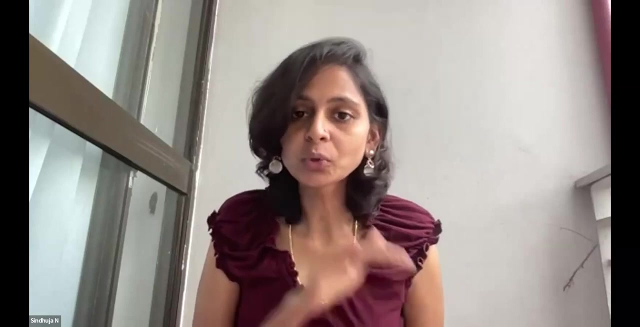 like our alphabets. You are, we are all writing paragraph, but we are not sure how the vowels are making notes right. So, similarly, if you're not clear on the software development lifecycle and its process, definitely that going to be a little bit challenging and tricky. So this video helps. 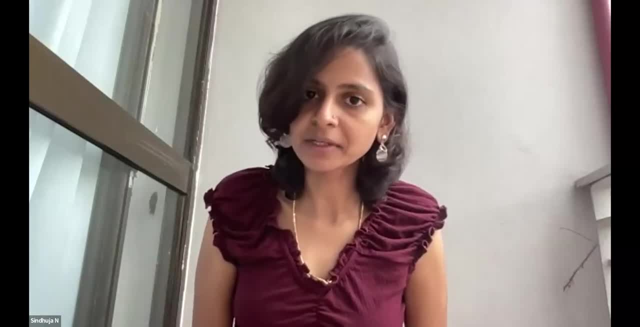 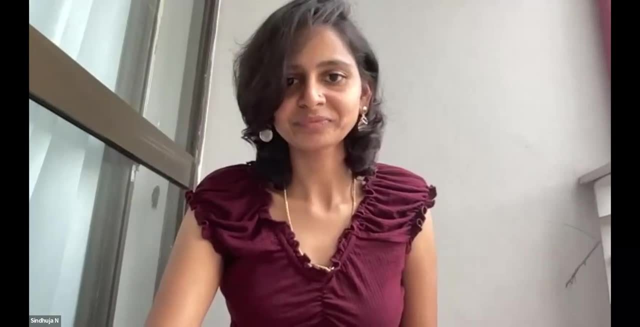 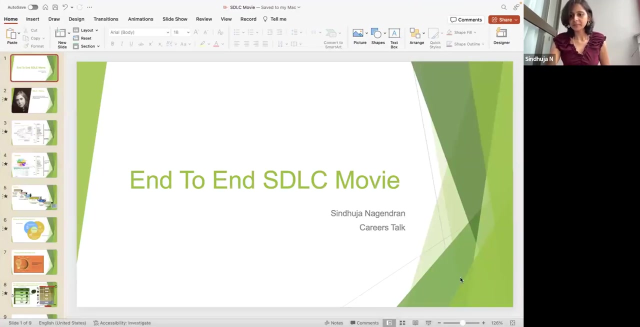 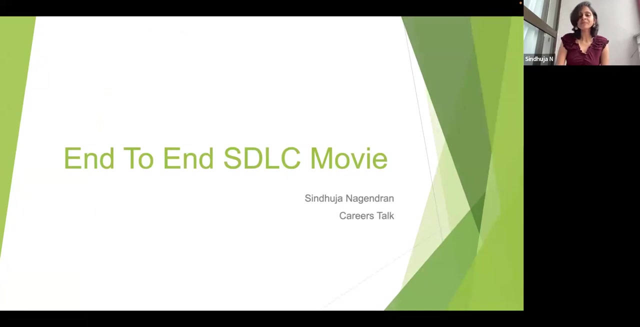 you to understand The complete picture of software development lifecycle, from the beginning till the deployment. Okay, so let's begin. Let me share my screen quickly. I believe you can see my screen. Let me confirm. So yes, it's end to end SDLC movie. Why I mentioned this is a movie, It's not just going to be. 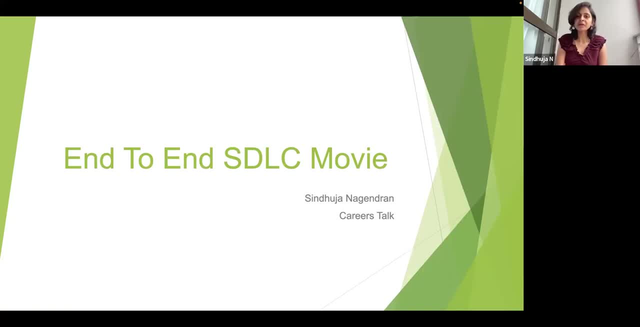 with PowerPoint presentation. I have made some mind mapping. It's a mind map as well. Some pictures are there, but I'm not sure how much I can take you guys in this short video, So let me try to put it up as much as I can. 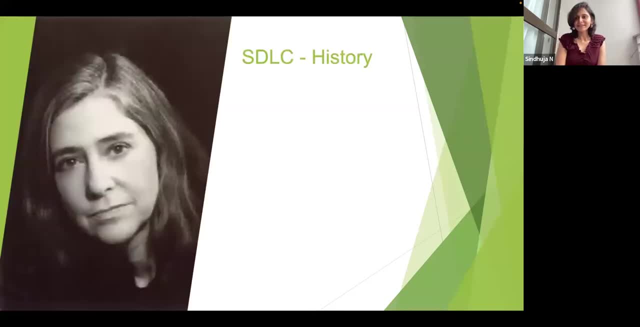 Okay, No, Okay, Let's start. Yes, How many of you are aware of this lady? By this time, you must have guessed someone or otherwise. if you're not guess, stay tuned in this video. Let me explain you. Let me tell you who is she. 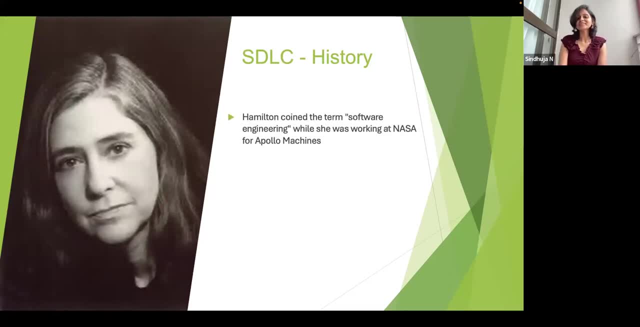 If you know, do comment in the comment section. So she is Hamilton who coined the term software engineering while she was working at NASA for Apollo missions. When she coined this term, she by herself, in one of her blog- I was going through. 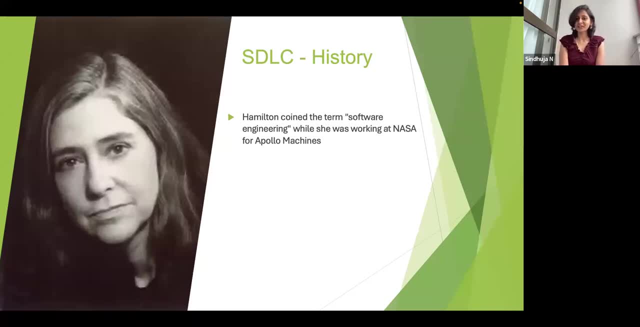 So many people made fun of her when she coined that of what does it mean, the software engineering? but she was the first software engineer and she coined the term software engineering after that. It's not happened now, It's during some hundred years ago. 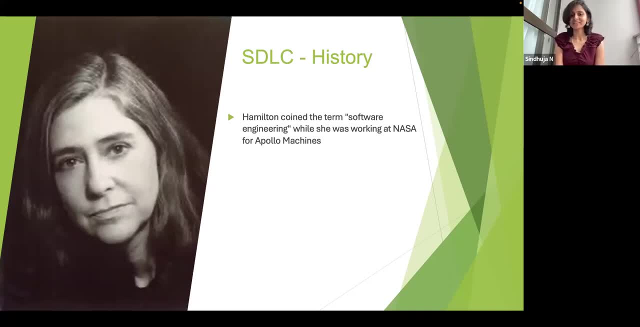 19.. No, sorry, 18 something, Not 19.. Even that time period. So she was a one pioneer, if I want to say, who was thinking this things and this kind of industry is going to emerge that time she started this one. 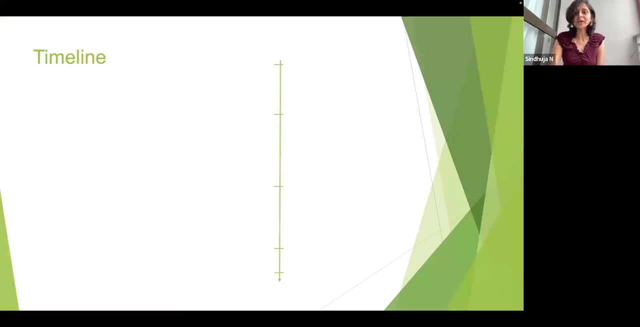 So her name is Margaret Hamilton, Okay. So let's see the timeline, how every methodologies okay, how every frameworks emerged into the market. A little bit Overview, Uh, completely Okay. So I'm going to give you a little bit of a tutorial for believing. 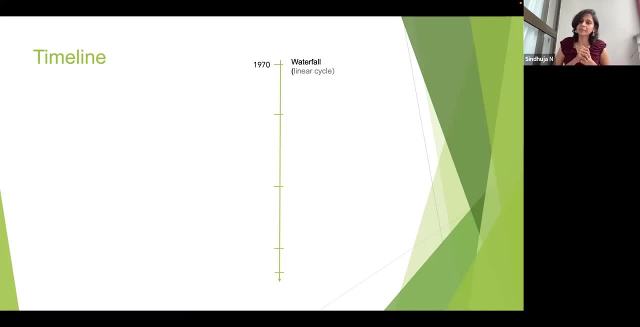 Okay, Okay, Let's start up So 1970, it was a time period where waterfall started to have. Okay, When we are always talking about traditional life, SDLC or traditional life cycle, we always talk about waterfall. but more than waterfall, we have many things in the market which 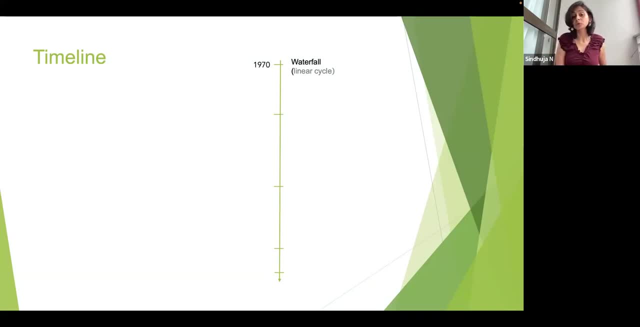 which is not maybe quite familiar or may not may used by many people or many organizations or many projects. Okay, waterfall is very common and we all know we always compare waterfall with ajal. okay, so waterfall is emerged in 1917. we all know how the way waterfall is. it's completely on linear, on planning analysis. 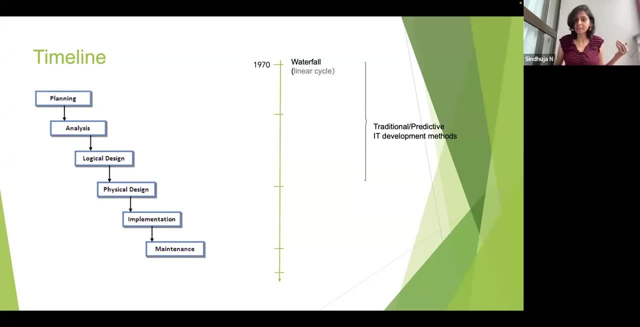 logical design, one by one, one by one. physical design, implementation, maintenance. this is how it goes: one by one, one by one. so usually the traditional method is always is so-called. it's not always, it is so-called predictive or it development methods. okay, so when someone use 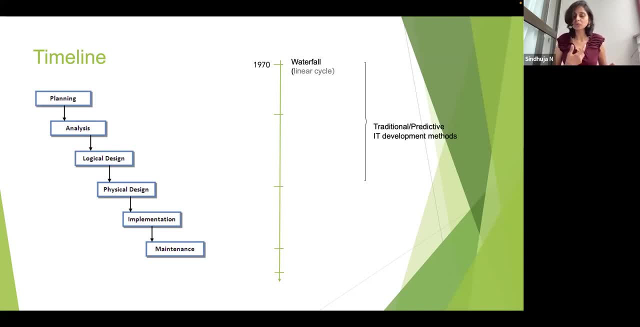 the term predictive- don't get confused in your interviews or whatever it is. traditional method is also called as predictive method. okay, so next to waterfall rad, this is rapid application development. many may have heard it about, but few may not even. in fact, for me it was new when i was. 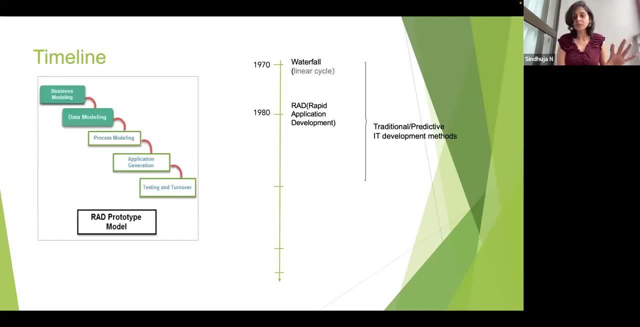 going through- and i was making this thing up so rad is some some other traditional model. it is also kind of linear style, one by one, one by one modeling prototype like that. only it, it has taken place. and then v model. v model is something common i believe many of us must have. 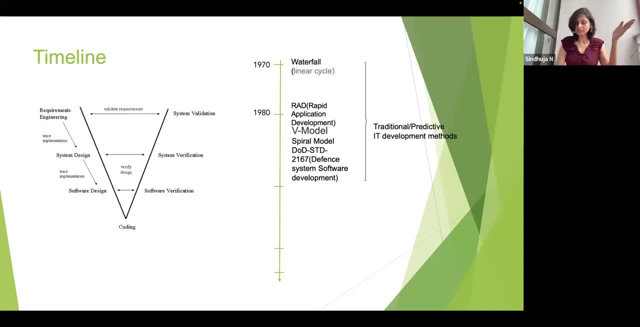 heard about it and this is our v model, so it will start the way it has: shape v. that is how it it starts up. okay, so it will go like d and then take a peak again and then the spiral model. this is also something we must have. 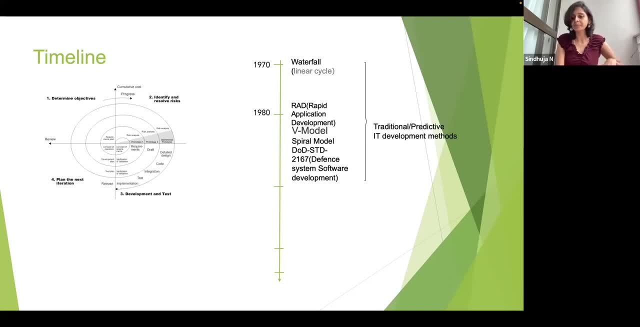 heard about it. so spiral model also goes in a loop kind of thing. okay, and dvd. this is something pretty new for me, to be honest, which i was so surprised by reading this and get got a chance to discuss this with one person. so this is something specifically designed for a different 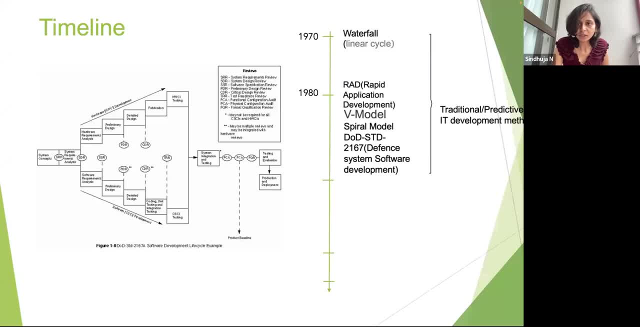 system software development. if i want to elaborate this, if you see closely here every phase, how many requirement reviews and design reviews, many reviews are going since it's being developed for the defense thing, the review and the rigidity of this test which i feel, which i felt it's very good because it's something secured and safe. 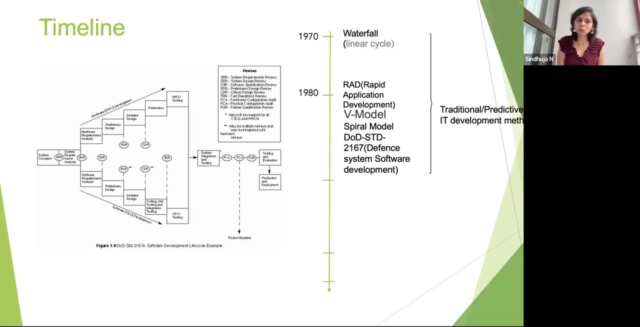 they are ensuring. so dvd std 2167. this is also another one software development life cycle, mostly on the american defense system software. they have used it widely- not now- during the time period of 1980s. so this was pretty good when i was going through and reading these blogs and everything. so the 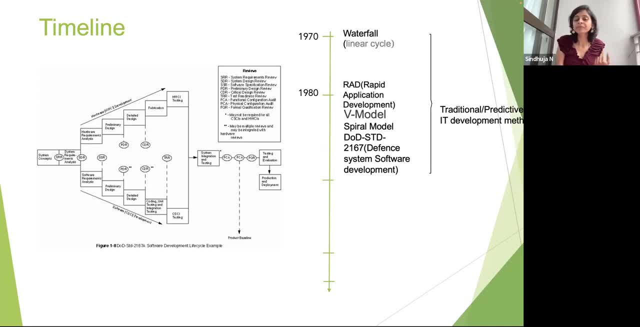 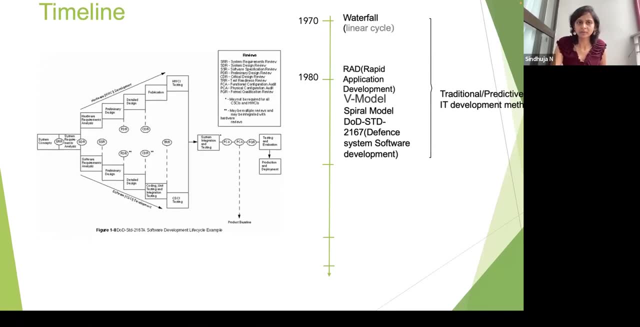 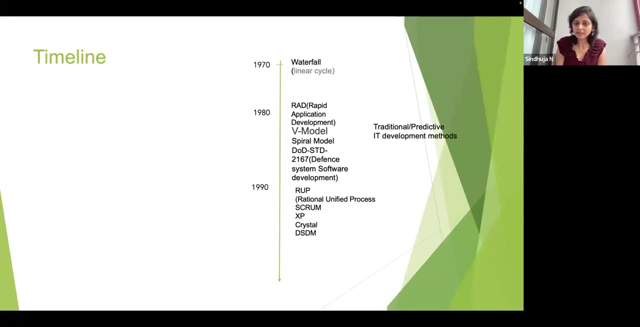 review system, stringent this process and ensuring the safety and the reliability of this one. okay, so moving on to the next slide. oh, i'm not able to move. i think i'm making sure, okay. so next thing we want to move: 1990s, and um, um. 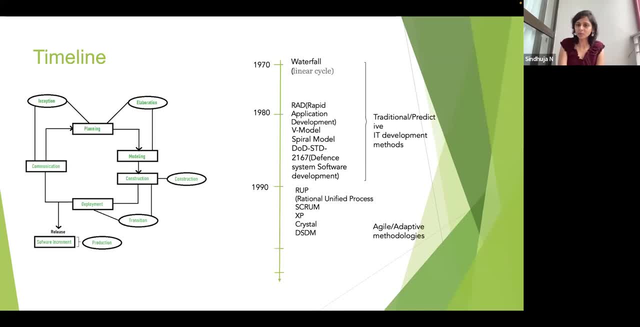 model one second. so root this is another one thing. but this is not coming under traditional or predictive development methods. it is coming under agile or adaptive methodologies. so root model is rational unified process. that means this is an iterative model. this is not like how our waterfall works. this is also an iterative model. it goes in an iterative incremental process. so this is true. 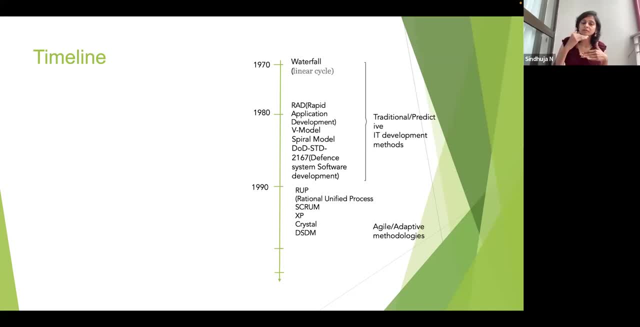 rational, unified process. so this is an iterative model and this is not like how our waterfall works process, which, which is which came ahead before scrum and scrum framework. pretty much we all know what it is and how it is. and then xp: i love xp a lot more than scrum, i believe i i sense. 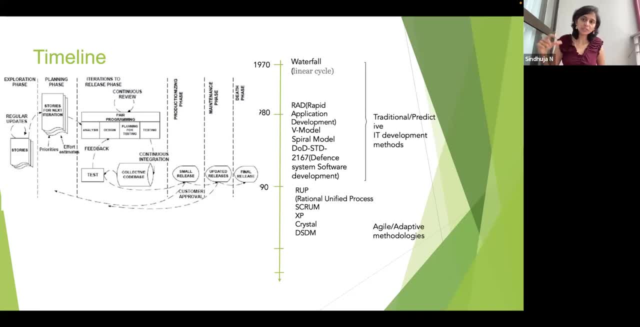 because most of the concepts, what we are using at this moment in the industry, thrives or evolved from xp, for an instance, if i want to say, even the user stories. okay, so that time the couples only came to this picture, right, they this user stories, that concepts evolved and emerged from xp. 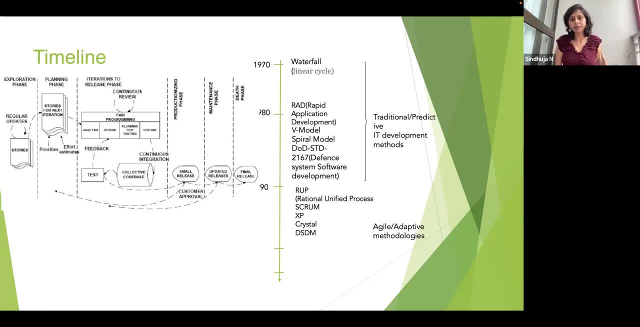 and pair programming. we are widely using pair programming nowadays to ensure the quality and cicd pipeline structures and everything. so this one, this continuous integration, these are all came from xp. okay, so, xp, we go with xp to ensure the more quality, extreme programming, extreme quality we will. 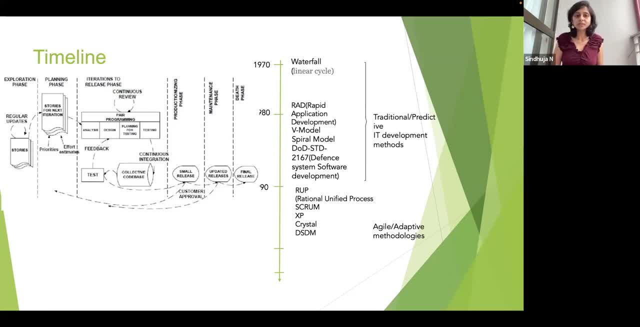 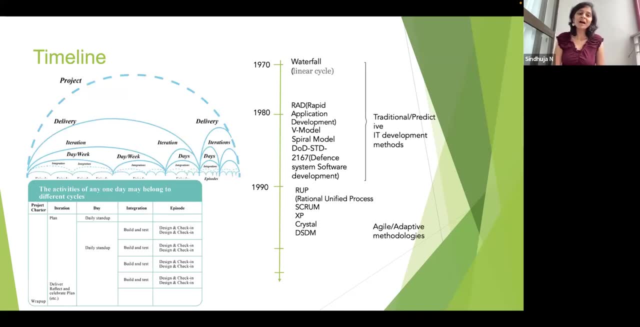 ensure that time only. we are going for xp. so this is the xp framework how it works, and crystal crystal. i- to be frank at a friend, i haven't used crystal. at least i have gone through kanban, xp scrum. i had a little bit of opportunities to work on cover on these areas, but crystal is something. 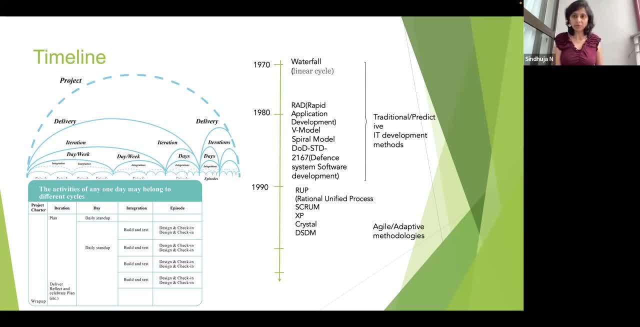 i never used, but still i'm looking at in many places in the job descriptions: crystal, you want to have some idea, but uh, i don't know. but still, however, i captured it and crystal has many things: crystal, yellow crystal, red crystal, team size, some colors. based on that, they have it. if someone is good at this, please do comment and educate us. 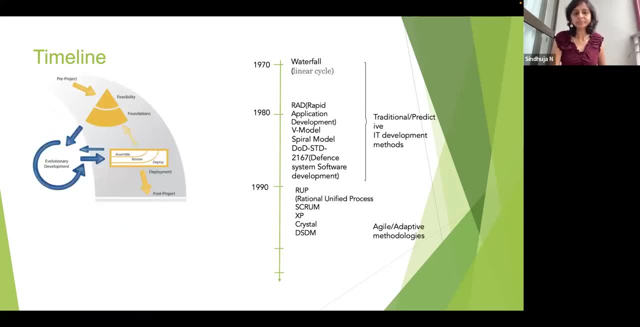 as well. and dsdm. so dsdm it was in the industry. nowadays, at least as far as my small knowledge, i'm not seeing this, but again, i'm not sure- in any in the other country, any other region, any other places or any other project organization or using this dsdm. okay, and kanban. we all know how kanban works. many must have. 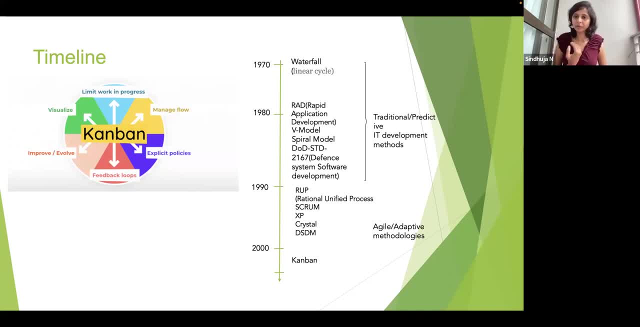 got a good hands-on experience incumbent, so kanban is also a kind of uh increment that's being delivered when the progress comes on to limit. work in progress with limit is one of the beautiful concepts in command and many other things right, okay. so this is, in short, about the. 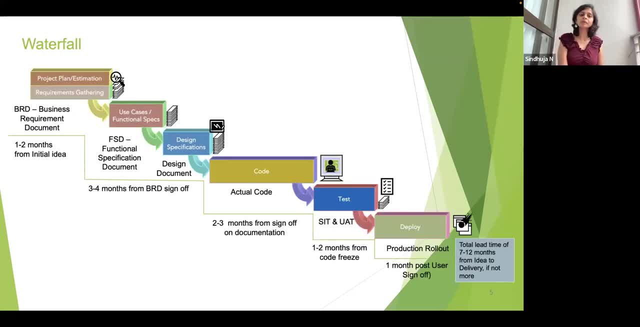 software development, life cycles, what exists in the market, okay. so, yes, the way we deliver software may get deferred, but the phases, what we are going through, must be the same. there is no differences like, um, without havin the requirement, we can start the thing. without understanding the project, we may not start the thing. and in testing also, if i want to say for 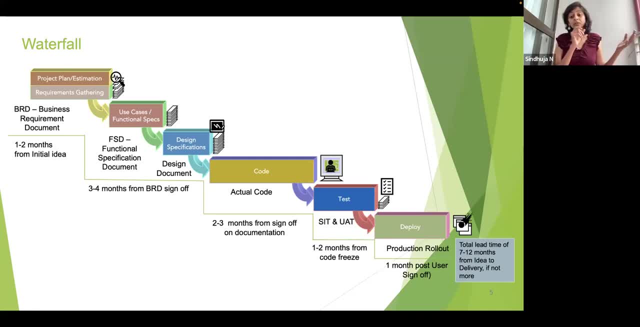 an example: the way we are developing or the way we are testing in the waterfall may be different, but But the same concept- testing- applies in Agile as well. So waterfall and Agile- the way we are doing- is different, but all the phases are going to be the same. 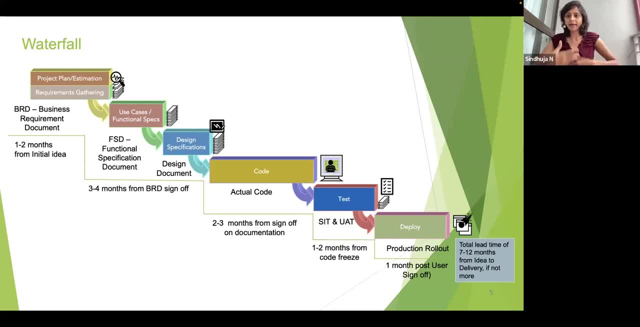 But the phases in waterfall step-by-step. in Agile it's go hands-on-hand, parallelly, right, But the phases are the same. So we are going to see what this phases means. what are all the segregations in this phases? okay, 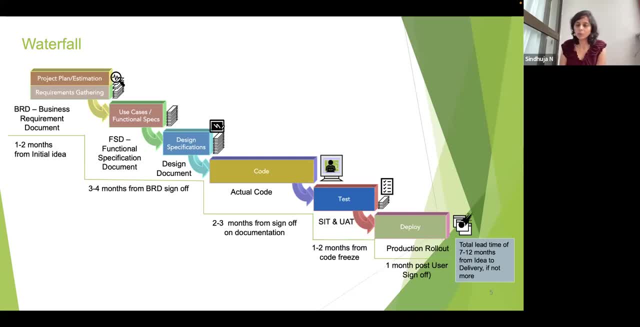 So in waterfall, in general we go with the requirement gathering or project plan estimation or something like that. But in terms of Agile, we will identify the customer need, along with the business owners or initiatives owners or stakeholders, whoever it is, And then we will come up with the inception meetings. 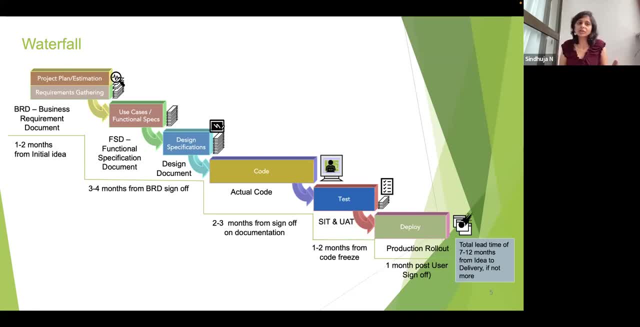 and we will derive the business process and then we will start right. So here business analyst will work with the customers and they get the requirements gathering. Once after the requirement in the design phase they will come into the picture of functional specification documents being prepared. 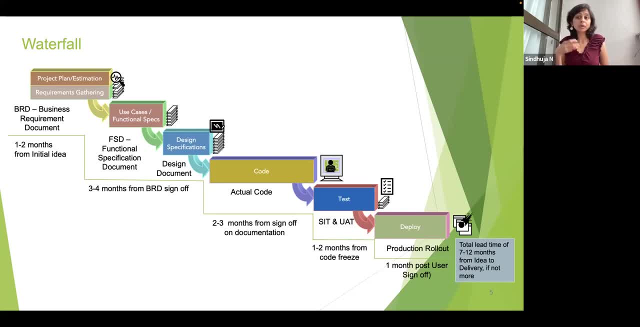 Guys, if you are very new to the software industry, when you hear the term functional specification document, don't feel like you lost something. So functional specification document is something which is being prepared in the design phase to let know. this is how the doc specifications. 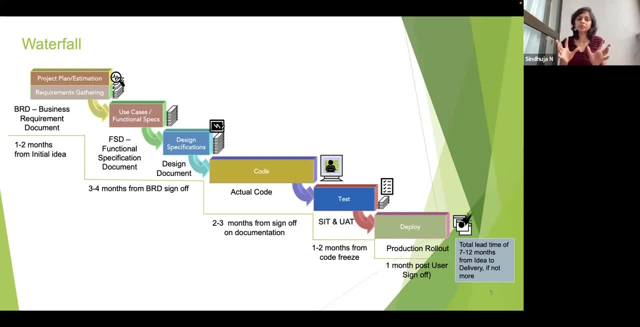 is going to be in a functional way, okay, So don't feel that or something they are discussing. So this design phase, it will be prepared, And then coming to the design document and coming to the coding actual coding phase will take. 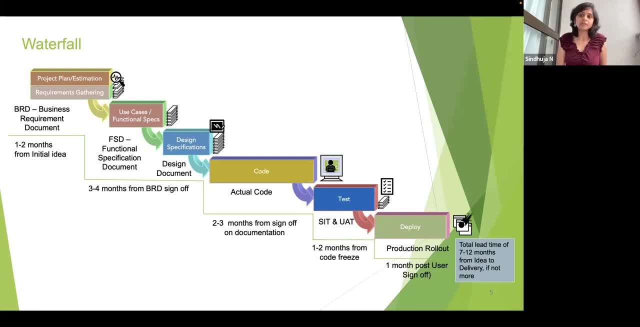 And testing, SIT or UIT, whatever the testing. Testing is again a vast area which I will show you today in our mind map, but still I cannot cover all the testing. but I will show you what are all the testing and the explanation maybe we will have. 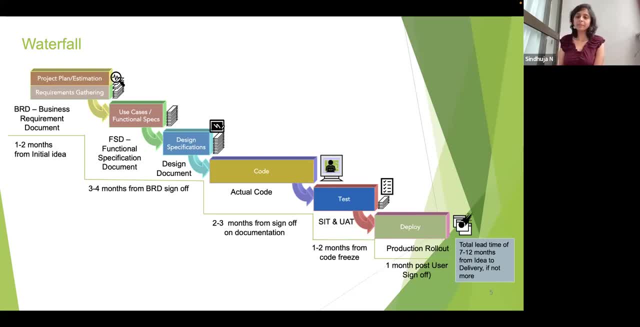 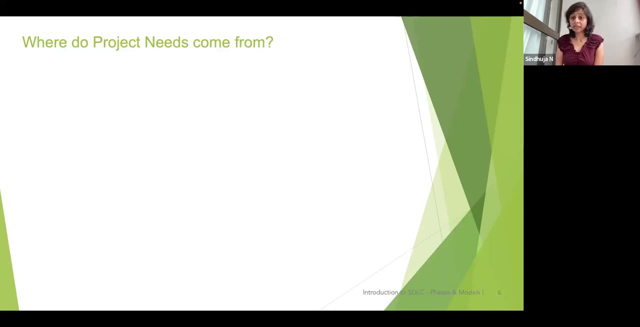 in some different session- And the deployment phase. then maintenance will come into the picture, right? So these are all the phases usually we have in our software development life cycle. Okay, where do project needs come from? before the requirement analysis: Many of us must be working as a scrum master. 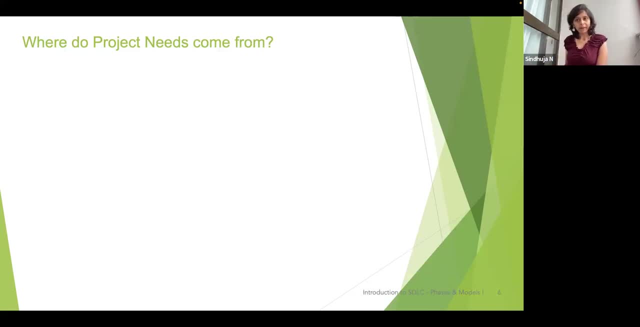 When we are entering into the team, we must have only the product backlog. We don't even know how this product backlog has been prepared and how this is being captured right. Where do project needs come from? Okay, the first thing: project or program or product. 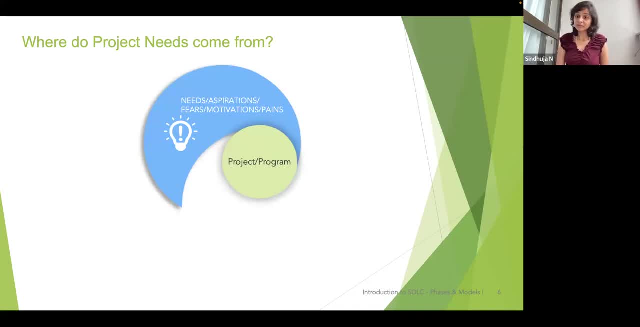 okay, whatever it is: needs or aspirations or pain points, fears or motivations, something like that. So that is the start point for us to get some project correct. When you have some pain point pain, then that time only we will evolve. 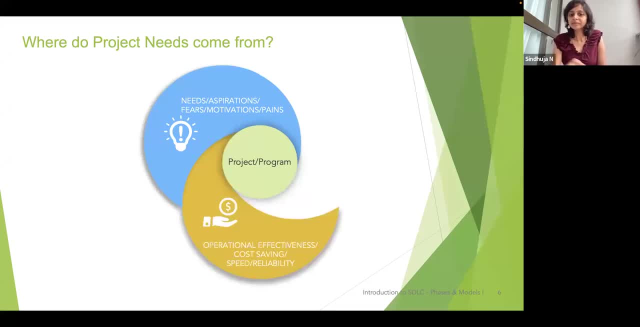 and we will identify many things. So that is the start point. And operational effectiveness, cost saving. If in case in your organization you want to scale up something, some inbuilt house project or internal projects must be there right, So that time and all we can use. 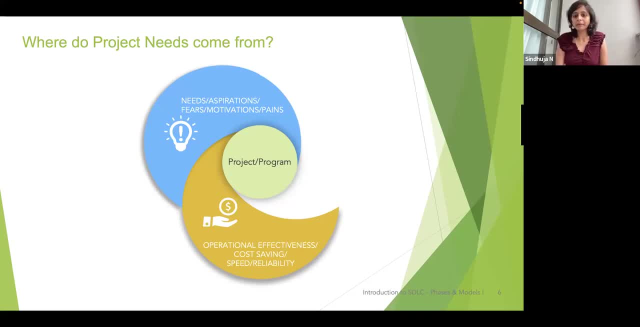 as operational effectiveness, cost savings, some internal development projects, these and all will come. So this also some kind of requirements. Another one thing is that the regulations compliance security audits. if you're working in the banking domain, more approvals you want to get. 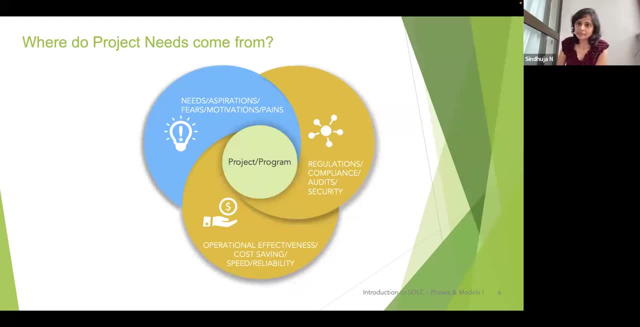 Similarly for the insurance. you want to look at the more compliance risk stuff and everything right. So this is how it is: the domain based on the domains. So if you want to build up something like this, then this comes into the picture of the requirements, okay, 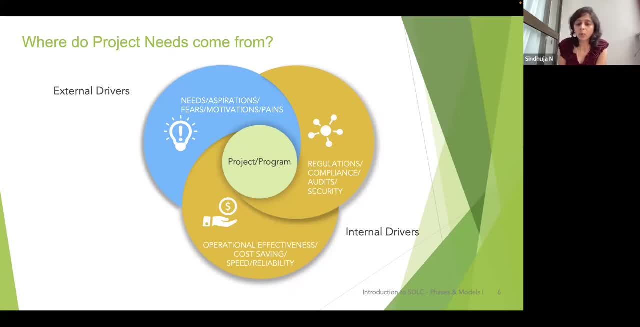 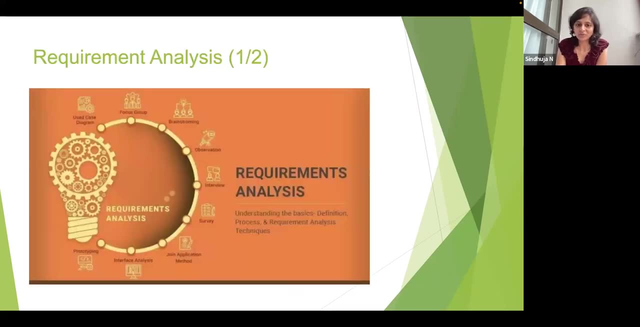 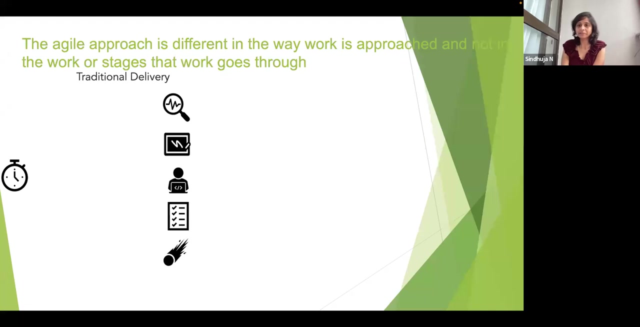 So the first thing is an external driver, the remaining two, the one in the yellow or internal driver. So requirements like this- Okay, I'm not going into this requirement analysis Maybe. So if I want to say the agile approach is a little bit different. 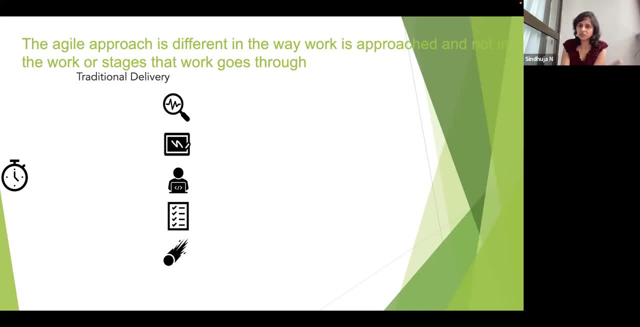 before getting into detail, I will just let you know how this traditional and agile ways of working is working. okay. So in traditional delivery we will go like this. okay, That means go like this in the sense, not vertically. The time will get elapsed, one by one. 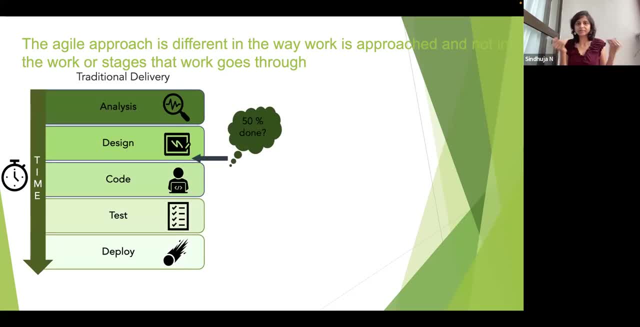 but we, we, we, we will go once after analysis, design code test. when we finish our design, people will say that it's 50 percentage done, or when we are finishing our coding, 60 percentage done. but in ideal, in reality this may not be the case. it varies, right, because we are yet to deliver something to the 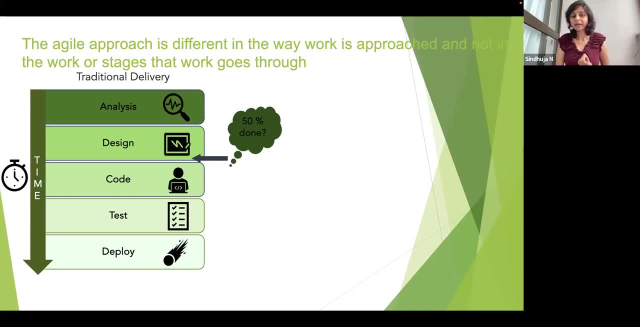 customer and get to know whether this is what they are interested. it may differ so, but in waterfall or whatever, the traditional methodology, either it can be v methodology or something else, so that time it will go like this time will get reduced based on the, the cycles, what we are going through. 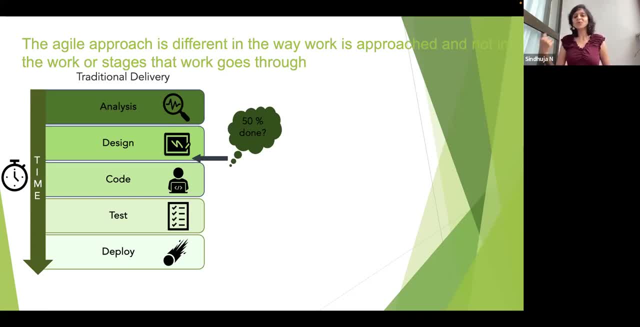 and we are going one by one. after analysis we will go for design and code and test. okay, but in agile, okay, like this, all together we will deliver. analysis, design, code, test, deploy like this: chunk by chunk, we will deliver. but in waterfall, analysis goes first, design goes next, like this: but here, if you see analysis, design, 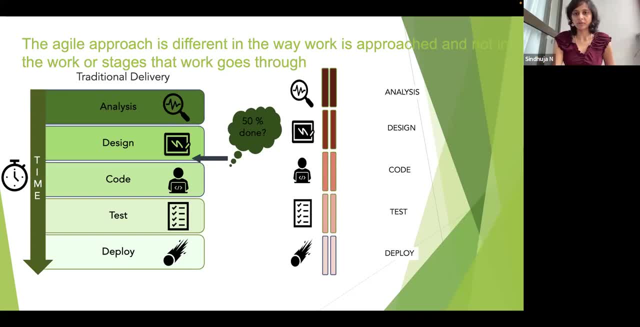 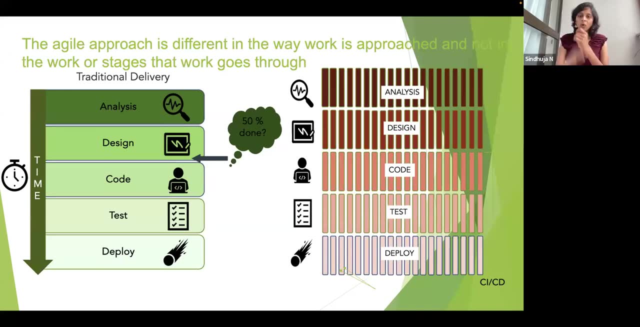 code. test is one phase, another thing, another phase. this is how it is. see, this is how okay. so this is the difference i hope this picture explains. we will go in a vertical way with the things. so by the time when we say the time will go like this in agile methodology, by the time in 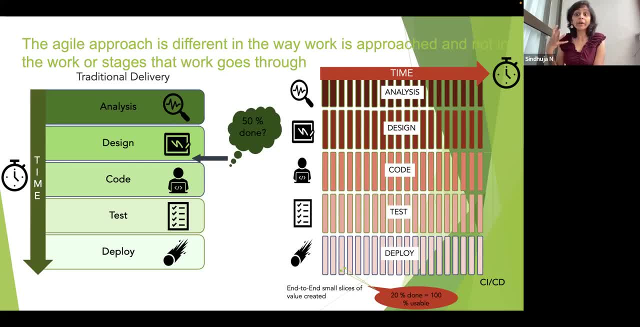 our third sprint, we will say 20 percentage done, that is equal to 100 percentage usable. that really matters. that point really matters. if you see in the slide, at last you can you know that yes, i'm 20 percentage only done, but it's 100 percentage usable at this moment. but the same thing when you say in the waterfall 50. 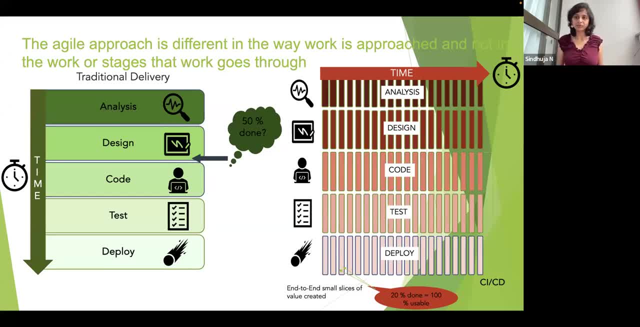 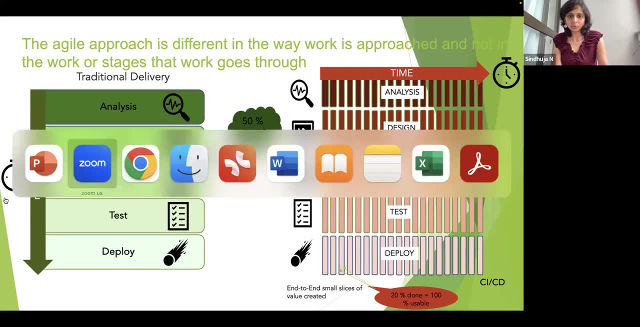 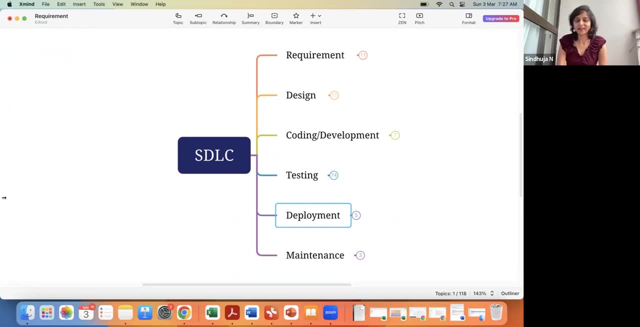 percentage done, it's not usable. again, it's like simply a key 50 percentage done, that's it right. so this is what the difference. okay, so let me take you guys to this mind map to explain what is stlc. so sdlc- again the same spaces i have iterated here: requirement, design, coding, development, testing. 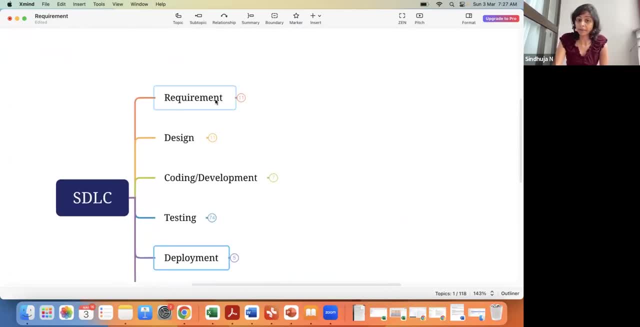 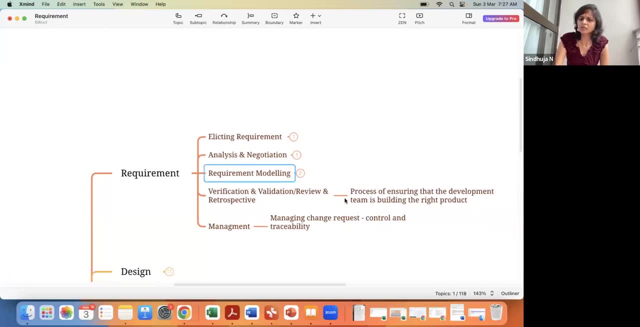 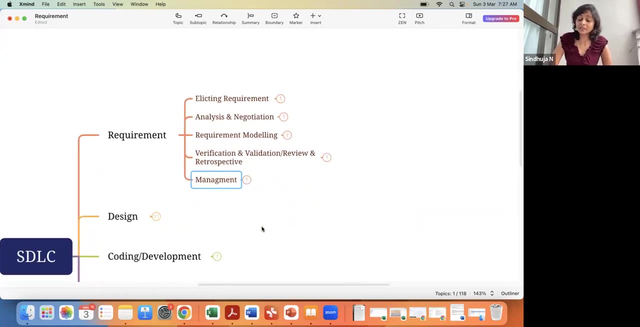 deployment and maintenance. when we are talking about requirements, okay, many things are there, but we knowingly, unknowingly doing many things, many things some organizations are skipping. it depends on the project. they are not even doing. so the first phase, or first thing, is eliciting, eliciting requirement, okay, so what it means. so the process is the process is the process. 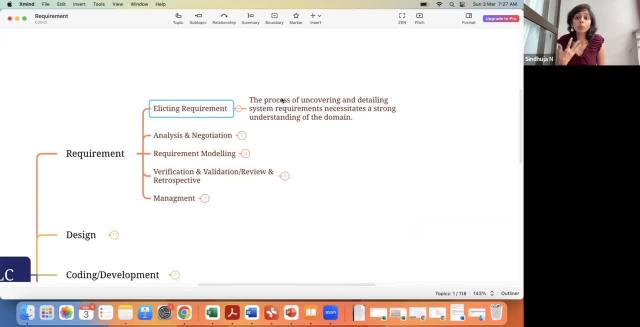 of uncovering. that means getting no more more about and detailing system requirements and necessity may be a business case, if i want to say necessity- a strong understanding of the domain and coming up with the why it is okay. so that is the first step: eliciting requirement. 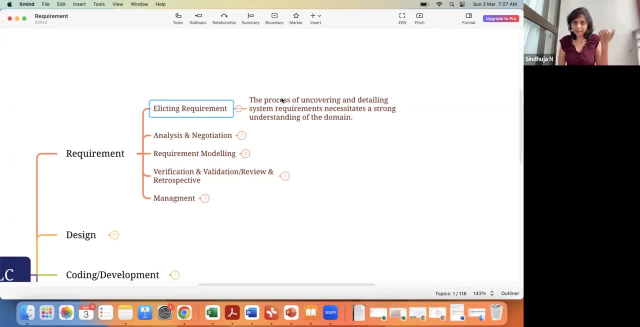 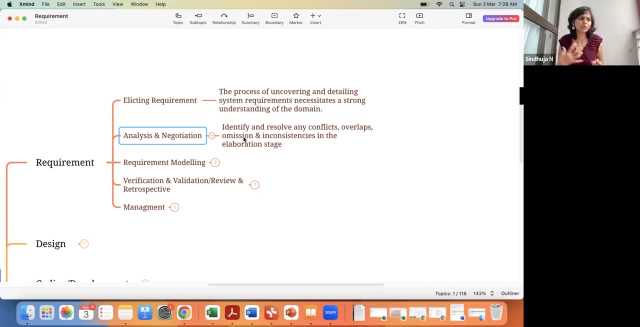 this is a step. this is how this is functioning- please use this kind of terms- going forward in your requirement phase or whatever the phase when you are doing it, okay, and then you can analysis and negotiation, identify and resolve in this analysis phase any conflicts or any overlaps. 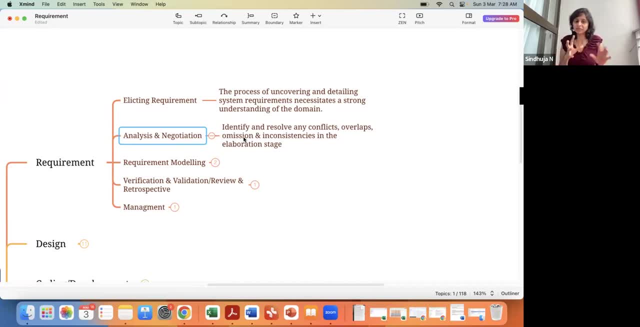 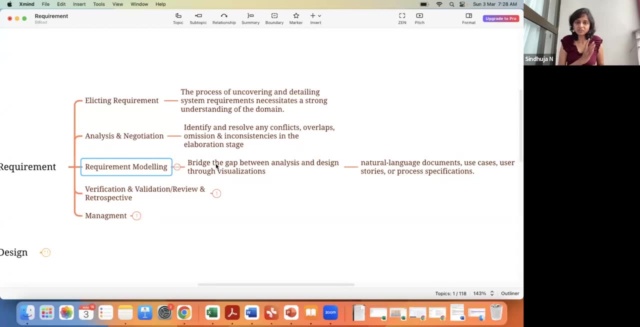 or any other thing. we want to consider this in this requirement phase, this thing we need to cover, and requirement modeling. so this modeling, what it will do, it will bridge the cap and between the analysis and the design phaser. okay, through visualizations, maybe a use case required use. 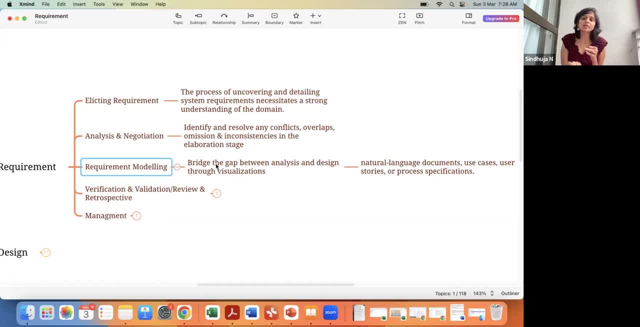 case red: writing user stories. if you are doing in an agile ways of working or process specifications, when you are writing the user case you use the stories. you must have had your business process flow in place in any other form, like any, any tools you can use to narrate. 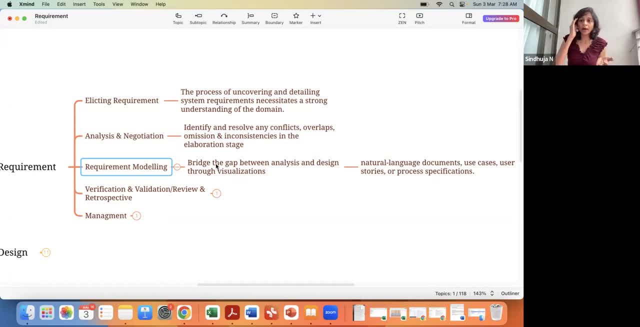 this one. so by that time you will be ready with this user stories. you have some picture, when you are working in this space itself, right, how it is going to work. this is what it is. so in the eliciting requirement, you are uncovering and detailing system requirements and necessities of. 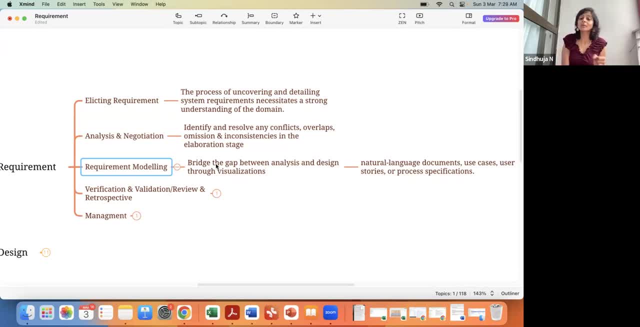 why it is needed, what is a pain point? so What is the motto behind this one? those things: Analysis and negotiation. we will identify and resolve any conflicts or overlaps. Sometimes some product: you must have built it Maybe, for instance, HTFC bank, mainly target on the salaried employees. 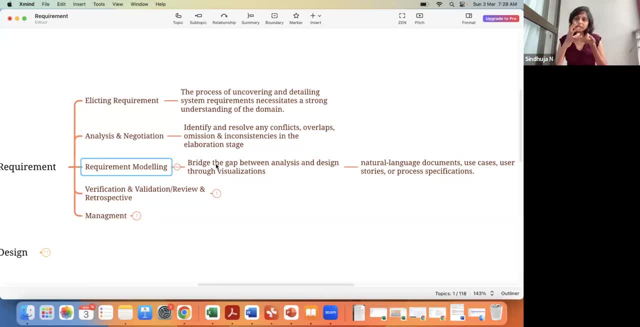 Their products are built based on the salaried employees, So in that salaried employees also, they will have some cross-cut categories as a middle-aged group, young people, parents like that. So if there is any overlap of this product, so how can we fix this overlap? 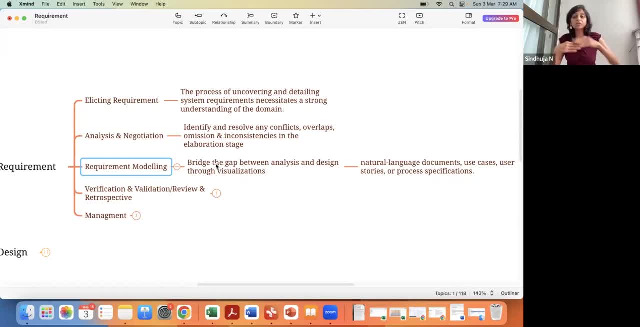 Something like that and all. they will discuss and analyze and negotiate and then come up with the solution or come up it's not solution again come up with the idea to whom you are working for this product, the personas and stuff. So this is a thing. 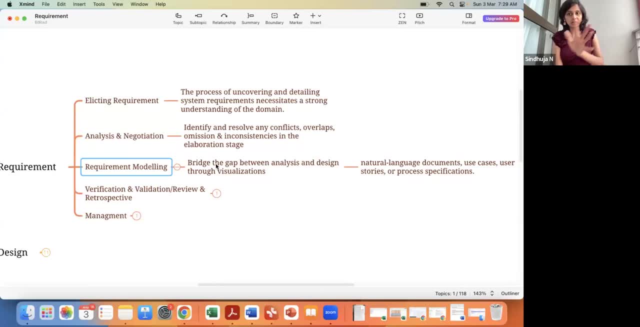 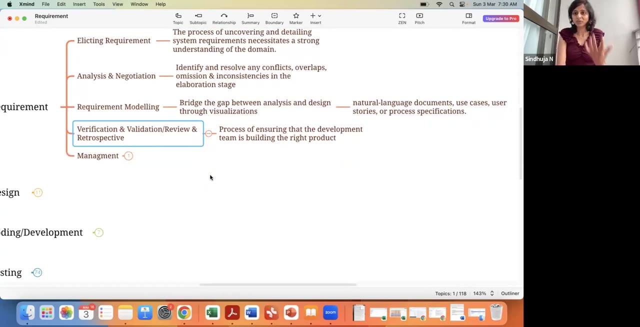 And the requirement, modeling, is that after a business process flow in our agile use cases, but if it is a waterfall, they are writing the BRE documents or some natural language documents, something like that: Verification, validation and, in fact, review Or retrospective, for all the same process of ensuring that the development team is building the right product. 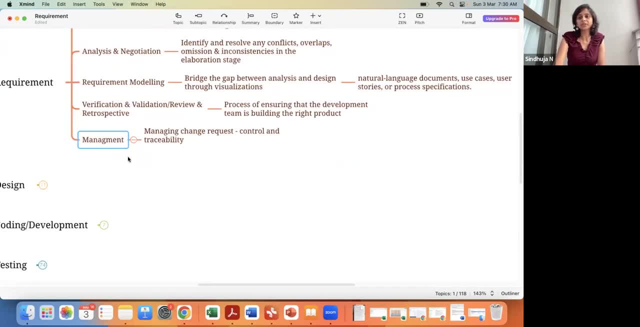 Okay, And then management: what are all the factors we want to consider when the development team are building the right product? That is, that is something we will capture in the requirement phase itself When we are doing our inception meetings in terms of agile. 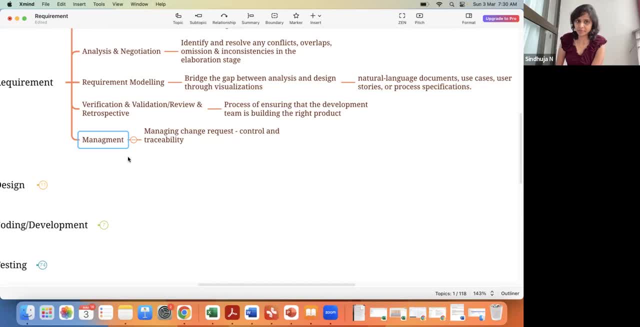 Okay, And management managing, change request control and traceability. Um, I should be very specific when I'm using this management term, because in waterfall, Once The requirement is for freeze and things, if some of the change requests are coming, it should be properly documented and necessary sign offs and necessary approvals should be in place. 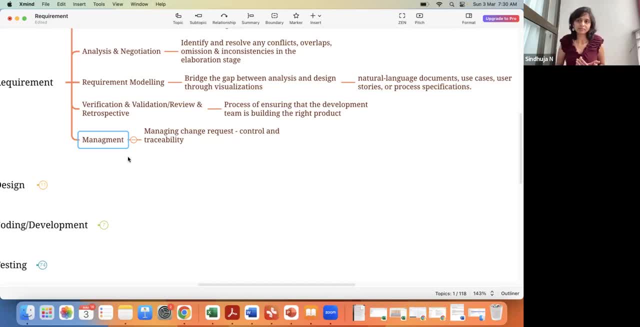 But when it comes to agile, we know changes are more accepted. Okay, But yes, of course we are also mapping it, but still we are happy to accept it And it's a frequent changes are expected in agile as well. That is what it is. 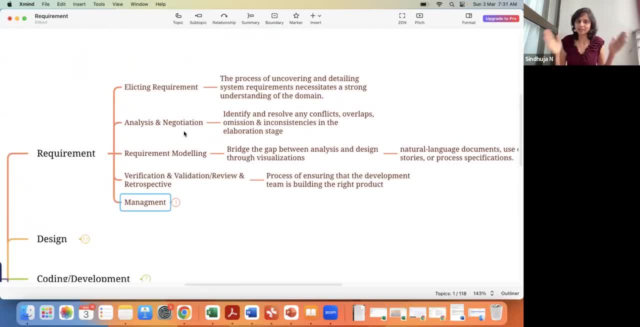 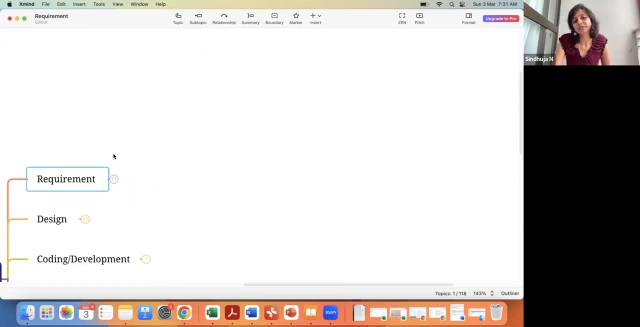 So I think this phases We are setting: requirement analysis and negotiation, requirement modeling, verification and validation management. So these are all something which is happening in the requirement phase. We may not use this terms in proper, in the requirement phases or something like that, but knowingly, unknowingly, we must have working in this space. 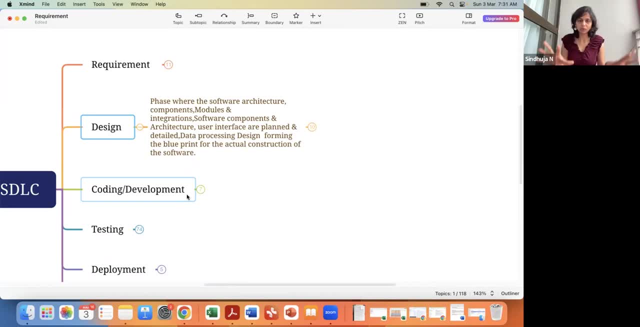 Okay. And design- simple, You don't want to read those things. Design is something where the software, architecture or competence, modules or Anything, any integration components, something like that. Here We will be having the blueprint like: how, if we want to construct a home, we have some blueprint to do. how okay, here, the kitchen should come here. 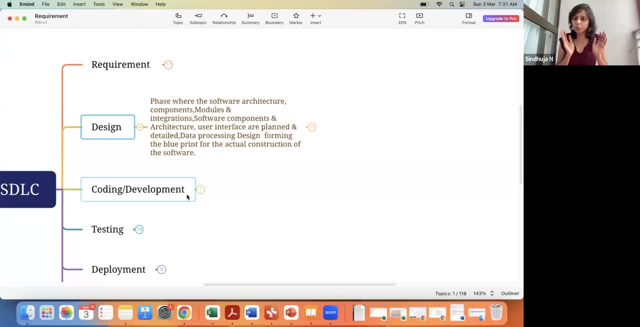 The restroom should come here as a master bedroom. that kind of blueprint It is. similarly, when we are doing our blueprint, everything, every input, every output, we will consider it. They suppose we are crossing the next person's Like that. that as well. 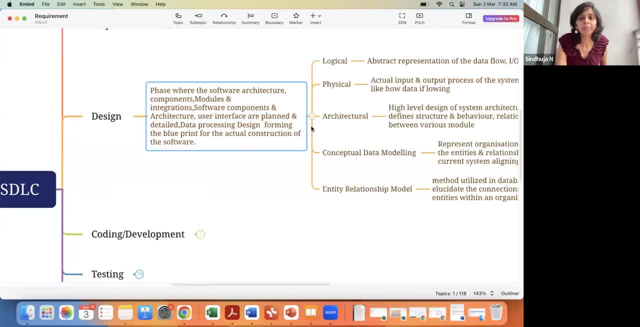 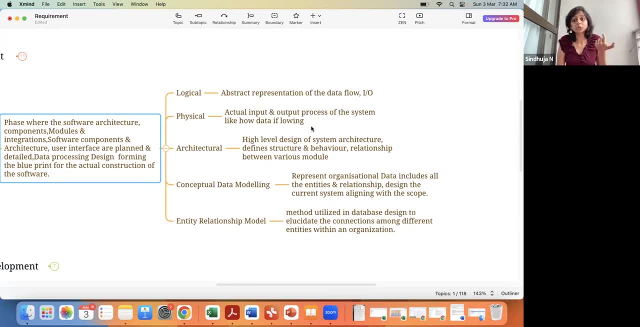 We will be covering And this one design. I think more than that, but in design phase we have a number of things which we may not have. a logical design, physical, architectural, conceptual, data modeling, entity relationship model, These are all things. 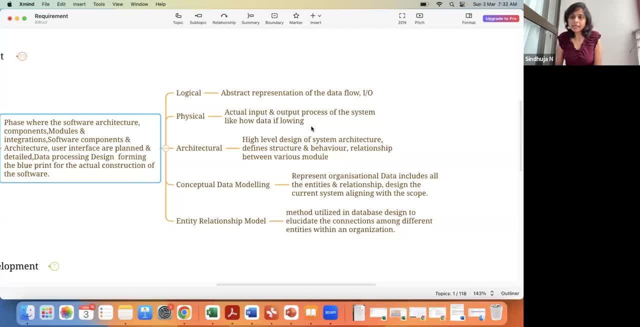 So logical is: it's an abstract. It won't go in deep and say it's just an abstract in book, Oh it's, it's just overview. Okay, Like how we are doing some research projects and all we do some matter for our abstract. first right. 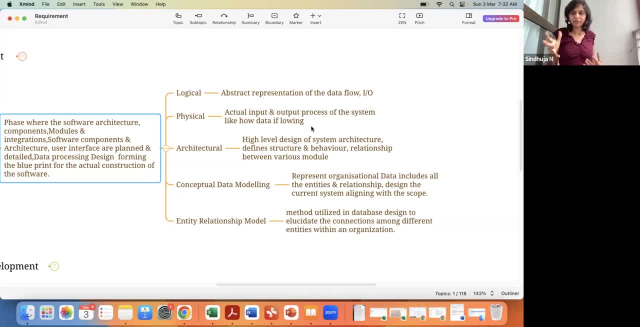 Even when you're Going as a speaker, we need to submit our abstract right. The same thing happening happens here: Physical, actual input and output process of the system, like how data is flowing. That is physical architecture, high level design of system architecture. 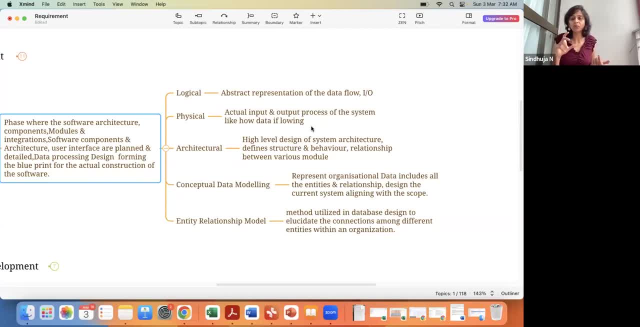 So this is HLL, where people will say high level design of system architecture, defining the structure and the relationship between various module. This is also something We really want to consider. when you guys were, when you in your team, people are using um some process. 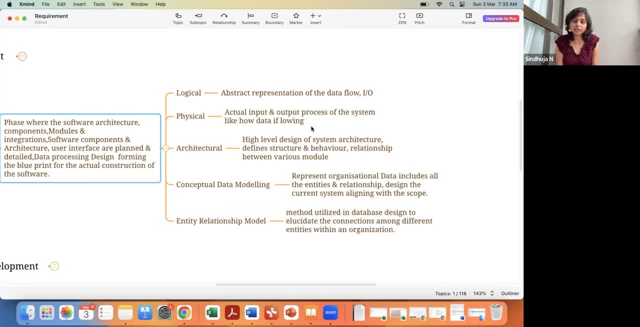 Okay, In your meetings or when you're designing a business process flow, that time people will say: this is getting the system, We need to touch the external system. This kind of topics will roll around. that time You need to consider, you need to know what kind of design they are stocking. 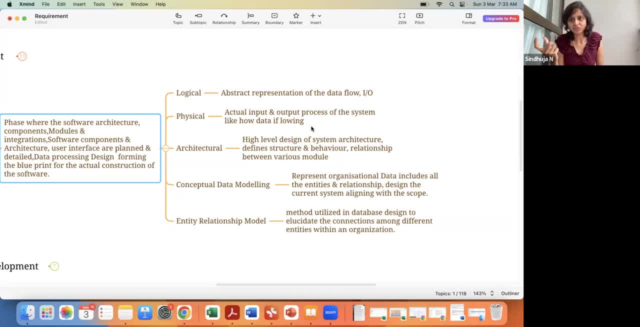 Okay, So what system it is touching? What are all the other modules? It is touching This, This is something being expanded- that architecture, conceptual data modeling. Okay, It includes all entities. entities I mean so small, small, small entities. 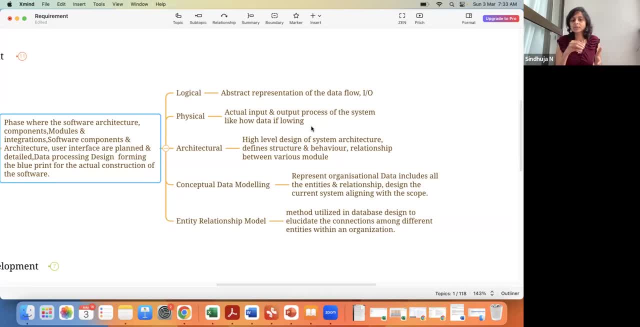 We must have need to finish up this project. So this is conceptual data modeling inside the organization. We will look at this. What are all the entities and relationship, Not only inside? sometimes we made the need to hit third party system, We made the need to hit our vendor system and internally. 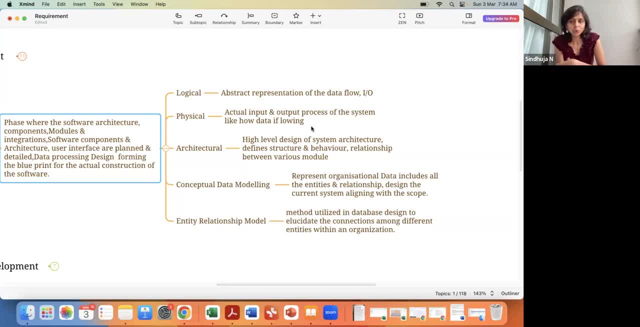 Some other projects, some of the systems. we made the need to hit it right. Okay, Done, Get the services, Something like that. Everything is interdependent with each other. interdependent with each other, Correct? So similarly, here in this conceptual data modeling, we need to look: what are all the entities this particular project or a program it's going to have our product. 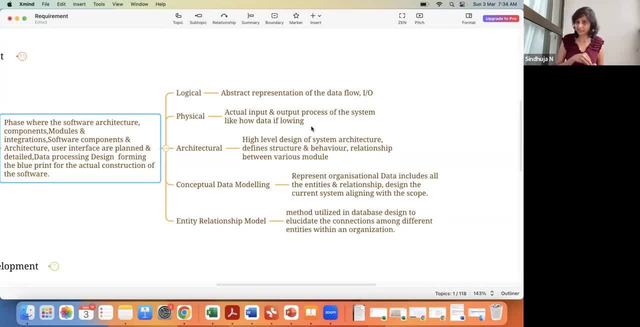 So that touch point we need to get. based on that understanding, we want to align with the current score. What we have, what are we about to develop? an entity relationship model is another one thing utilized in the database design. When, if you guys are a software- I'm sorry, database engineers or database those area looking closely on the backend of database activities, database activities, you must have heard about this entity relationship model, how each entity is relevant to each other. 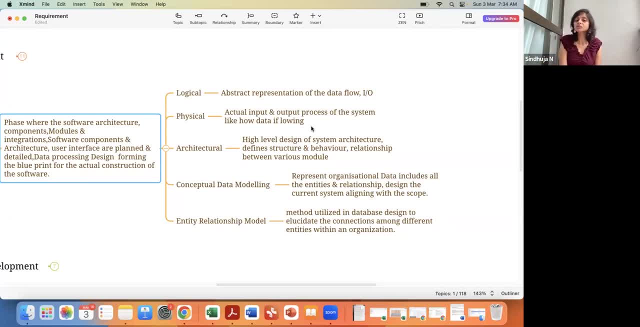 And the diagrammatic explanations will be so. this elucidate the connection, Okay, Connections- among different entities within an organization. what are all the entities? those things it will give you. So these are all the phases and these are all the things under the design phase. 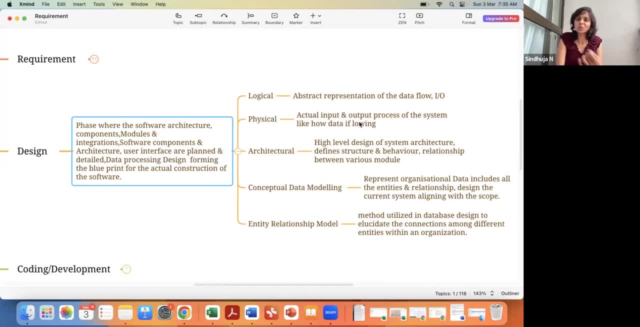 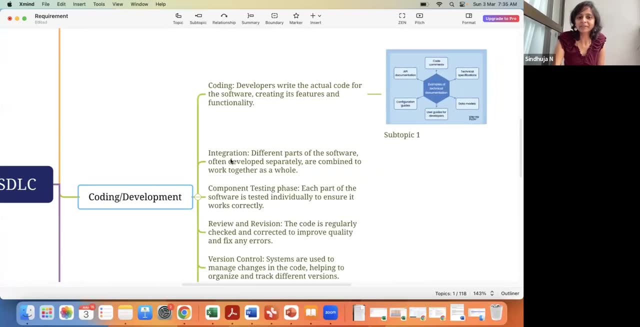 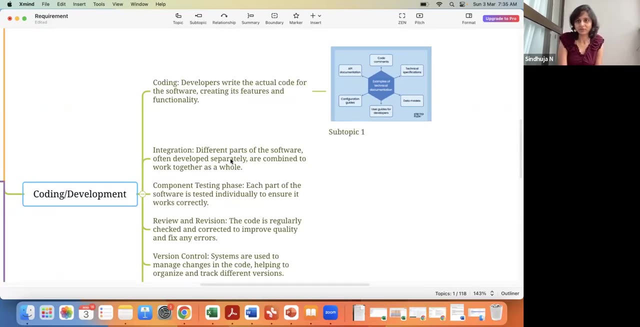 I hope it is a little bit clear. If you feel it's overwhelmed, pass the video and then go through it once again. Okay, So coding and development. this is something. coding Developers write the actual code for the software, creating its features and functionalities. 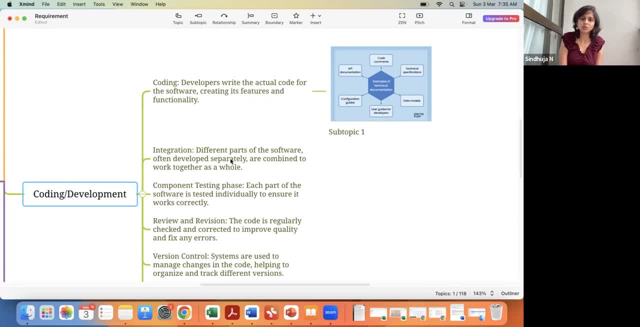 Actually write the code. That is what it is. Integrations. It's not just like being in a bigger organization or some product I'm developing, I just want to develop the coding. No, whatever it is, you want to integrate that with some other competence or some other modules or some other system. 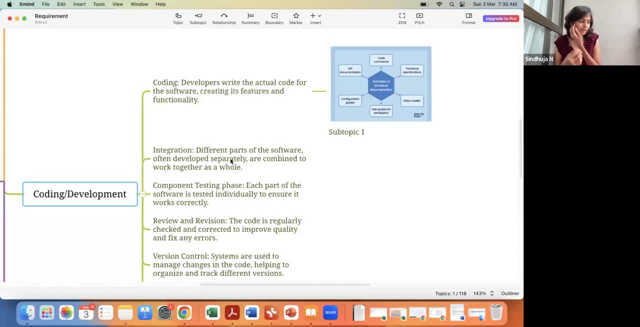 But if I want to do the banking, some transactions or something, it's not like I want to be insured with a source of funding Some payment thing, I want to payment domain or contract. I want to payment domain or payment tool or whatever it is. 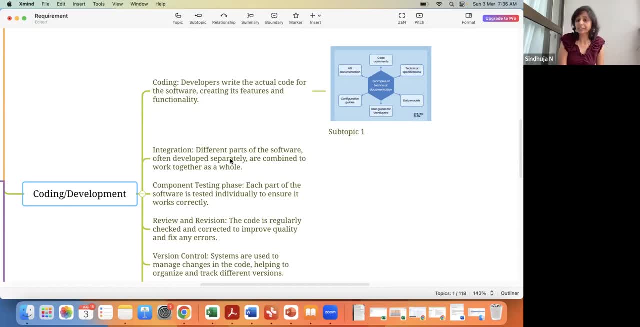 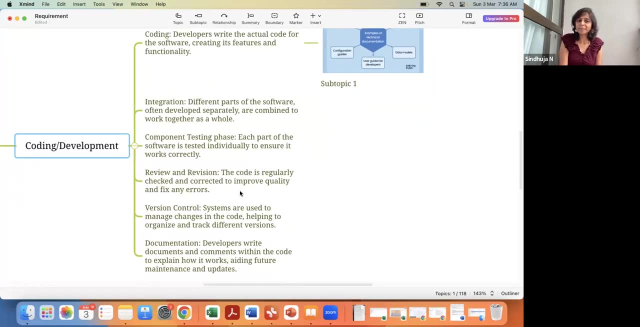 I want to tap with this, I want to integrate with that. That is what integration? So different parts of the software all tend to separately or combine to work together as a whole. Component testing phase In coding. Okay, So if you're new, please understand. 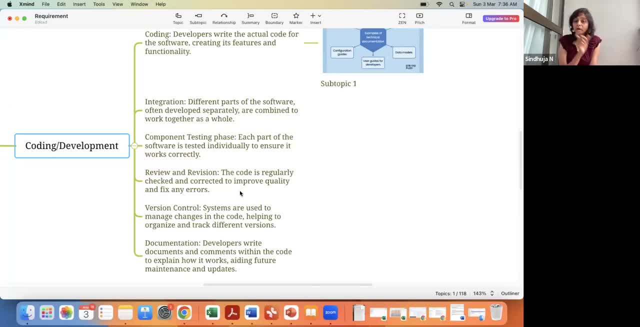 Testing has many phases, But when you're doing your coding itself, then that time itself developers will cover the unit testing functionality. That particular piece of code is working properly or not. Okay, So each part of software is tested individually to ensure it works correctly. 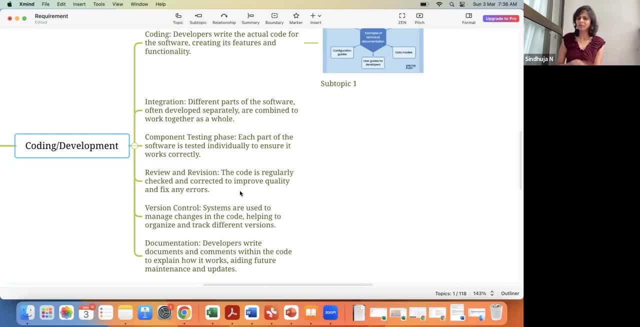 That is what component testing is: Review and revision In Agile terms, path programming. The code is regularly checked and correct and improve the quality to fix errors. That is what being used in Agile as a path programming And then version control. Yes, 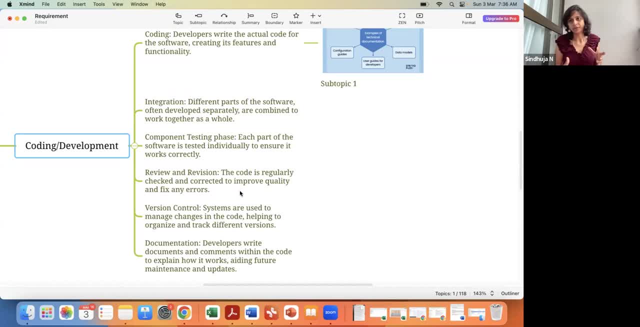 When you are doing your coding, you need to set up a version controls, CICD, Byte lines, Branching strategies- These things are not, But in terms of Agile, this is being taken care in coding phase in waterfall or traditional methodology. 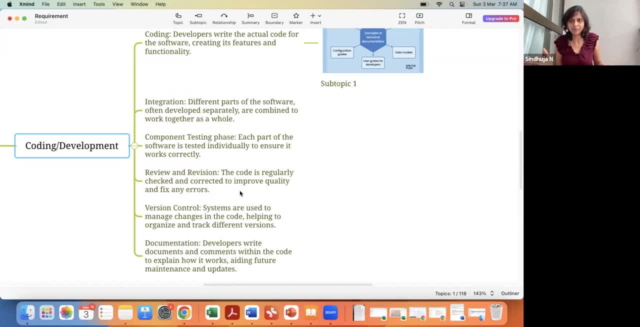 But in terms of Agile, before we start sprint one, we will set it up, this environment, Trunk based approach, if you want, Or CICD pipeline setup, Database versioning control. These are all few things we will do in our Agile ways of working before even our sprint one. 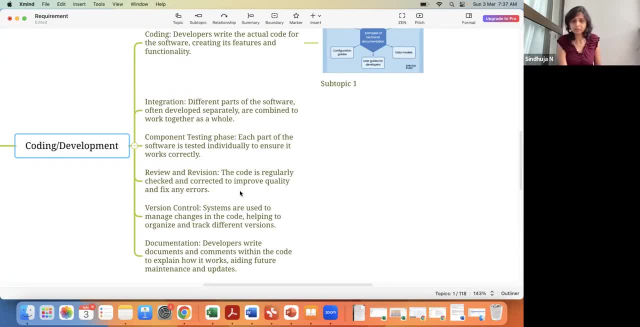 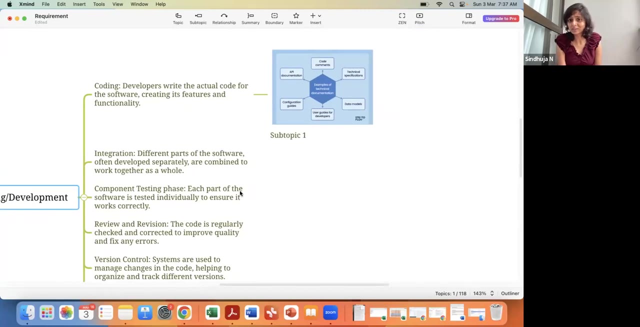 Okay, And documentation. So you may write some documents within comments, within the code, to expand how it works, Aiding the feature, maintenance and updates. So when they say this is finished, by that time only the coding phase has done. During your coding phase, developers may talk about API, technical specification documents, configuration guides, user guides, data modules, something like this. 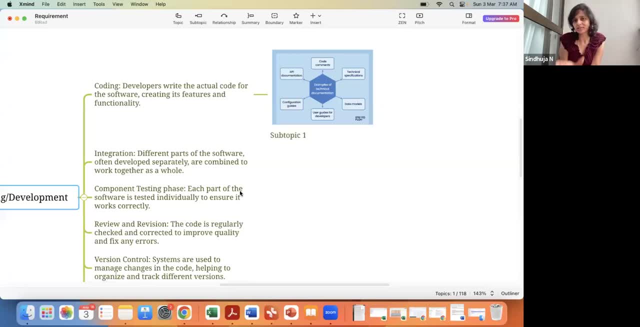 Even though you are a scrum master, you should have some basic knowledge and understanding of some basic technical stuff. You don't want to have over knowledge or you don't want to be an expert, But still it is always good to have some basic knowledge. 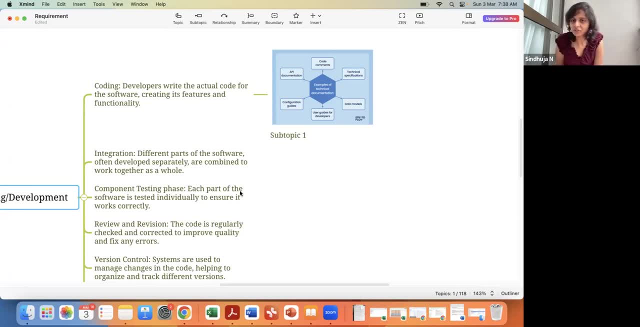 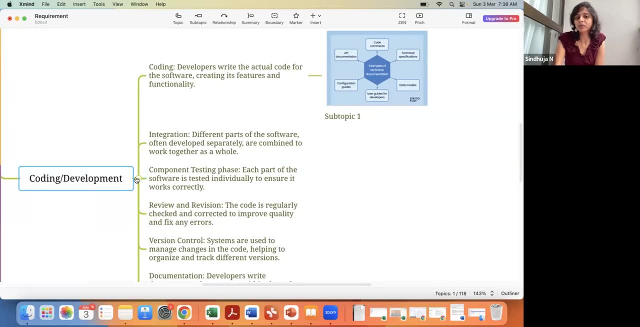 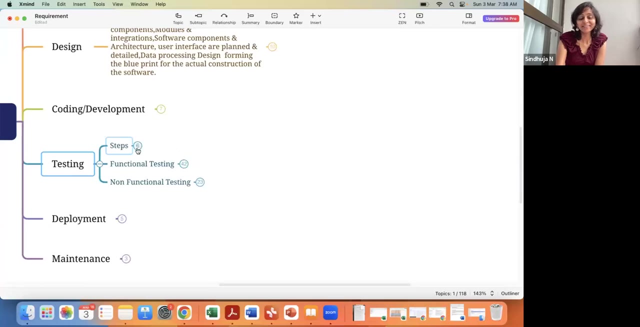 What it means by API documentation, What it means by API specification- So code commands, technical specifications, this things. So this will help you In this phase only. we will do all these things When coming to testing: 74 sub items are there, but don't get the 10s. 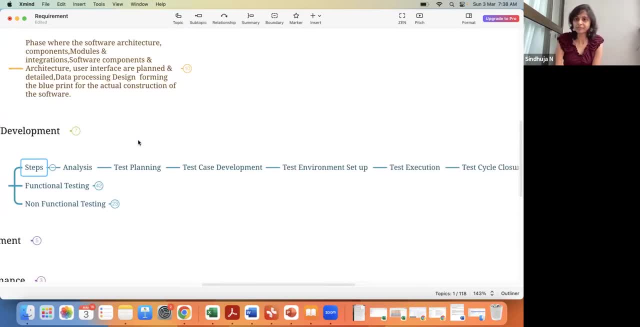 So, step by step, Okay For testing. The first thing is that analysis. They want to do analysis and they want to More than developers. I always sense testers should have the better understanding of the requirement. and why are we building this product? 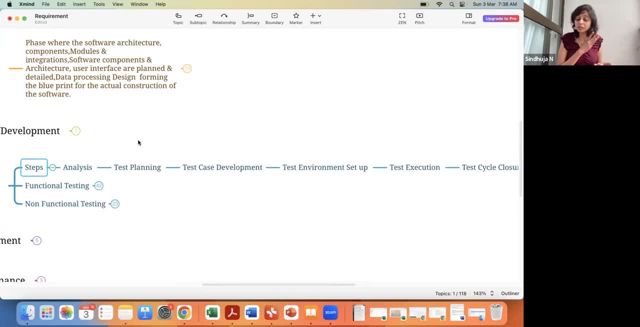 So if the testers have this better understanding, then things will be easily falling under their control. So, more than developers, testers should have a great understanding about the business, about the product, About the requirement. Okay, So, analysis, test planning, test case development, test environment setup, test execution, test cycle closure. 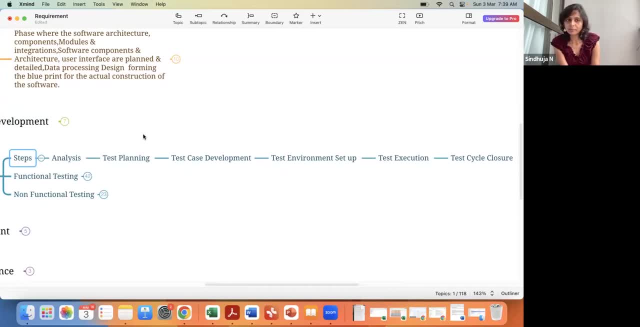 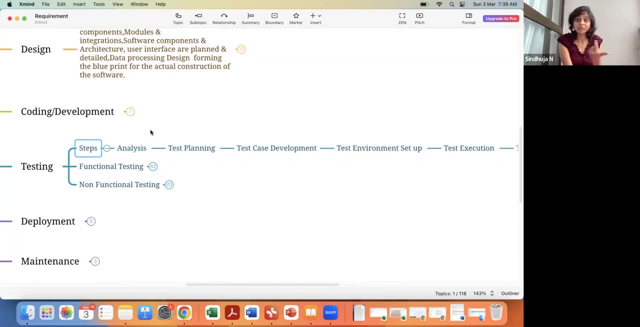 These are all the steps In waterfall, after the development or when the development is in the midway. testers started to do this: test planning and test case, development, environment setup and all But in agile ways of working. they will do it the initial time itself. 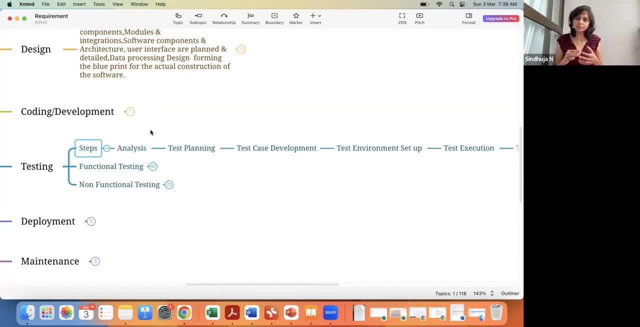 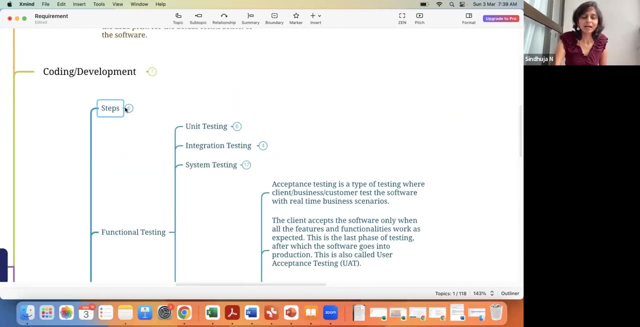 That means before sprint one, sprint one, they will do some basic environment setup or not. during the sprint one, when the developers start doing the coding, they will parallelly start writing the test case, development and remaining stuff. so okay, and functional testing, i'm i'm not going to get into each and. 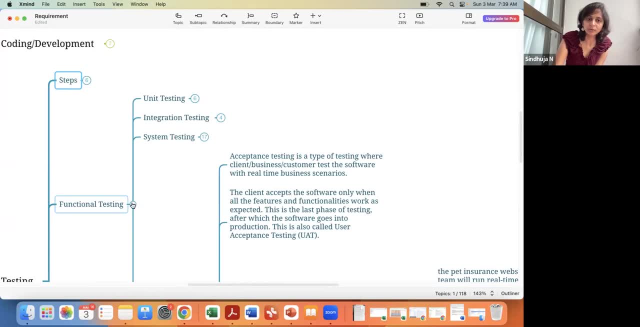 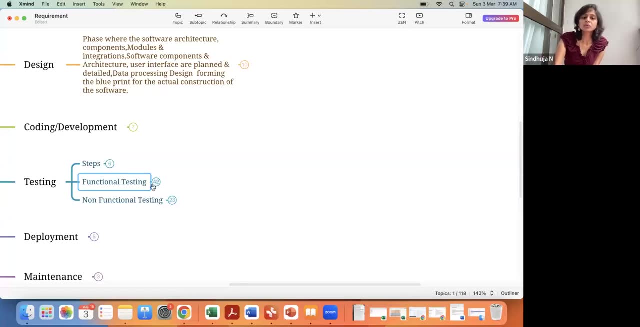 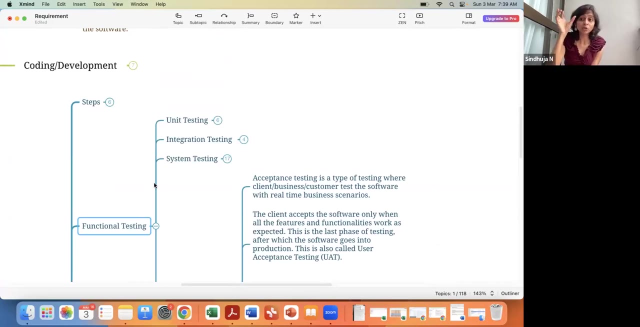 every pieces of functional testing, but i will let you know what is functional testing alone. there are two different way you can keep the testing: functional testing and non-functional testing. okay, so functional testing is something which will cover unit testing- which is which happens and which was which is being done by or taken care by developers- and integration testing. 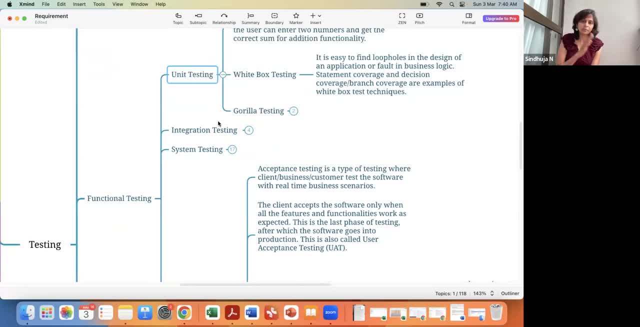 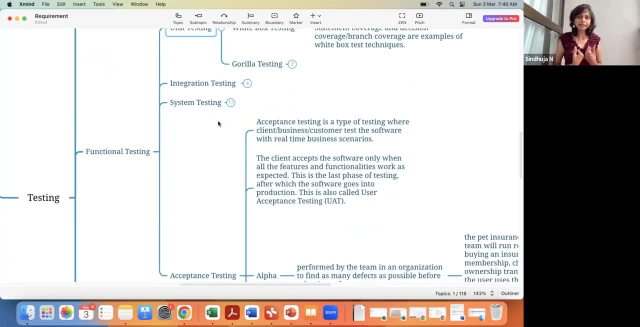 in unit testing itself. many things are there: white box testing, gorilla testing, so many things- but i'm not going into deep integration testing. integration testing is nothing. i'm building something and i want to integrate this with someone's system and that time it will go as an integration testing. 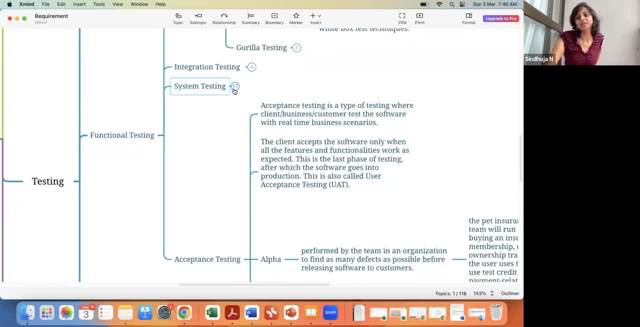 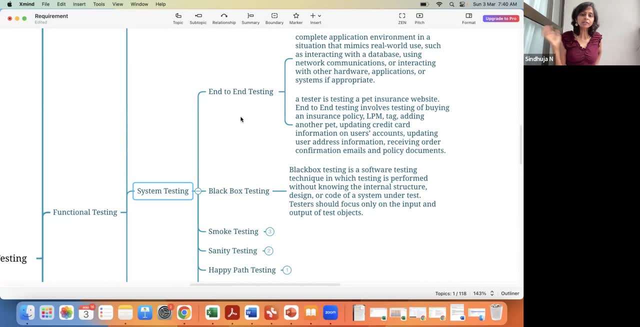 that is integration testing, integration and system testing. okay, so system testing is like end to end testing, but again it depends on the organization to organization who wants to go with what testing. black box testing, smoke testing, sanity testing, just a sanity check, light check that also can do happy path testing. 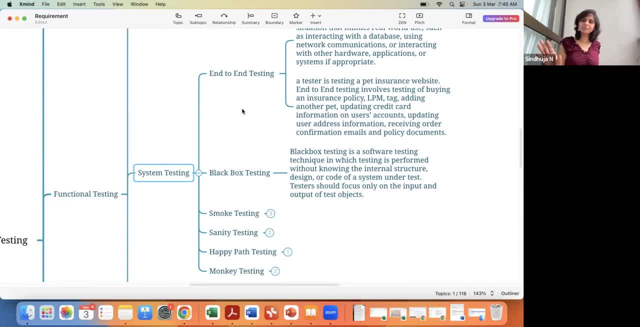 that means it won't cover any negative scenarios. happy path it means happily they will do like this is what the expectation. if this clicks, what happens? that's it. what if the question is not at all in place? what if the customer? or what if the end user? 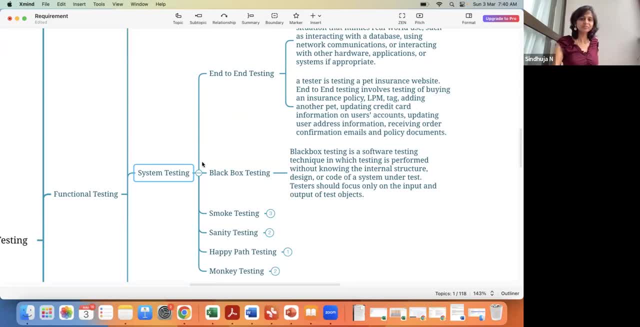 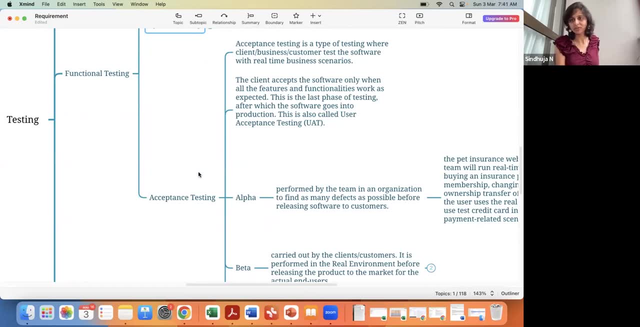 clicks this one, it won't come into the picture system testing. okay, so acceptance testing. in agile we always hear user acceptance criteria or user acceptance testing. so this is something uat, uh, business or customers will test and let us know where are we standing and what is the. 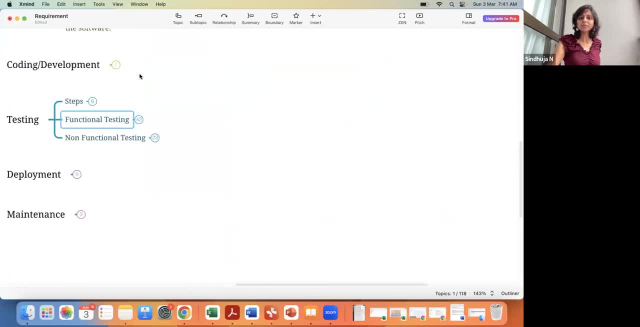 feedback. this is acceptance testing. okay, so there's a lot something under functional testing. one thing i really want to say here is that how much of our functional testing is important. the same way, our non-functional testing is also really important. okay, it's not like how much we are earning or getting into the market and improving our salary. 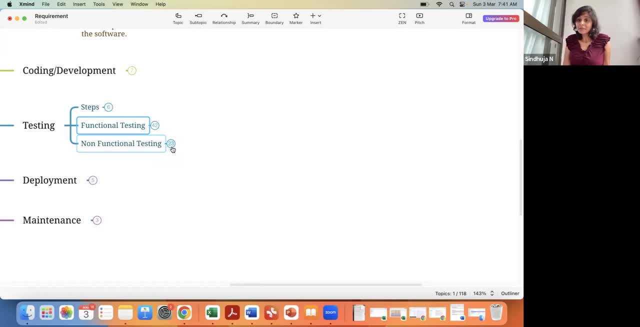 this is our function. we are doing it and making it. similarly, our managing our money. this is also matters. if you are earning, earning, earning, but we are not managing our money. what is the point of it? again, we will always in the need to work and we will be running behind money. so this is a similar thing. functional testing is. 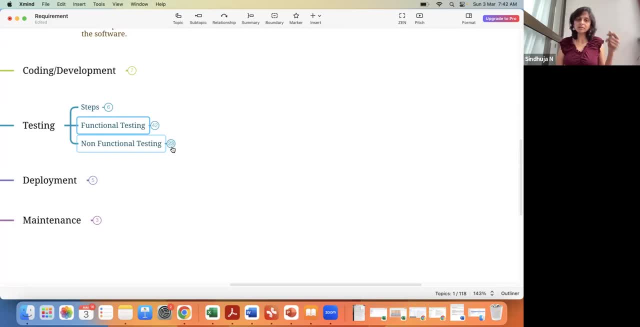 something which covers on the features and the development or whatever it is. non-functional testing is a supportive system which really we want to focus otherwise. so whatever we are developing, whatever we are doing, will be based over a period of time or will not be very productive, even if i want to rephrase it. 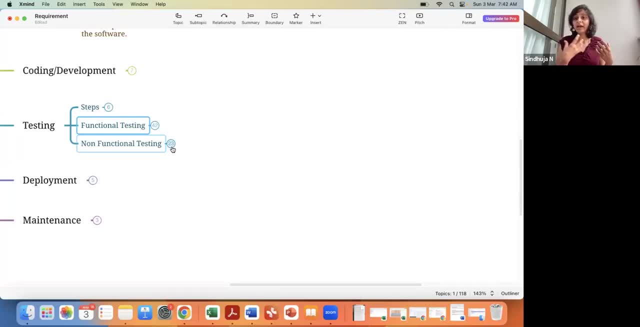 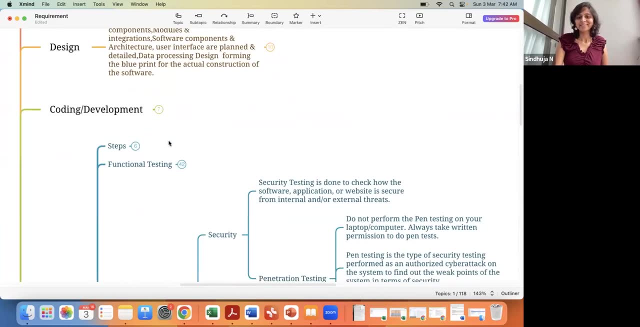 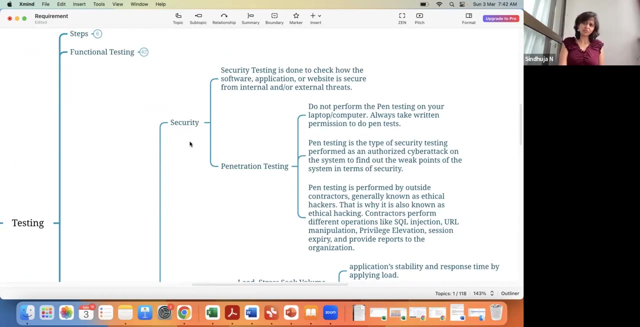 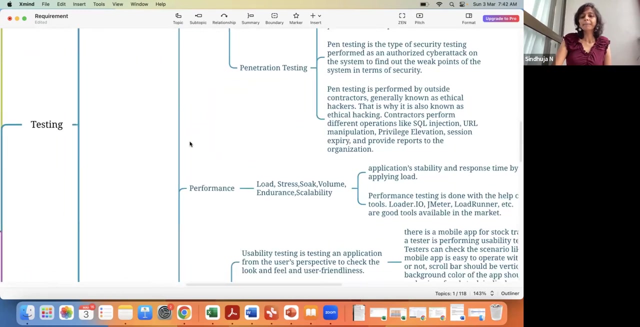 based. it may not be very productive and very helpful. it will be out or out of sync. so non-functional testing security. so under security we will come. penetration testing will come. few organizations are picking up penetration testing. few organizations are not. depends on the business, depends on the product, depends on the requirement: performance testing performance. it means it can. 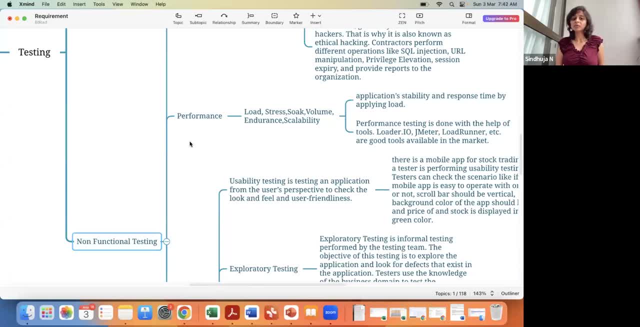 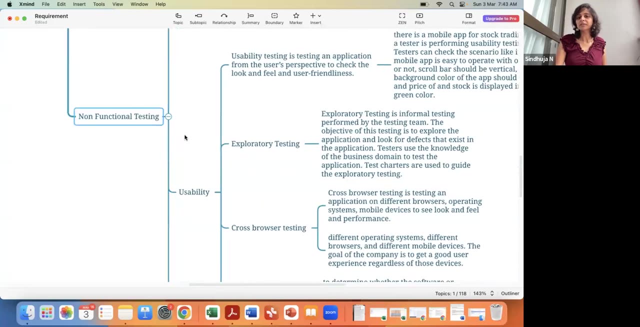 be loads, stress or volume endurance. this is what i said. you are earning lots and lots, but you don't know how to manage your money. you don't know that performance will be degraded- okay over a period. you will get stress- okay- and usability. so usability testing is the testing under usability. also, how frequently a 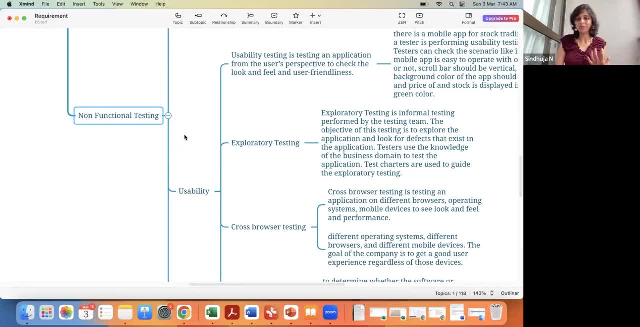 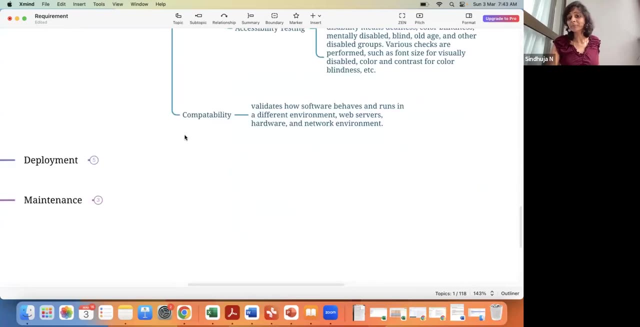 user's perspective. it is user friendly. that kind of testers will be done: exploratory testing or cross-browser testing, cross-device testing like android, mobile, ios, mobile chrome, internet explorer, safari. this kind of testings will happen under usability testing: compatibility- how it is running in different networking environment, how compatible it is. 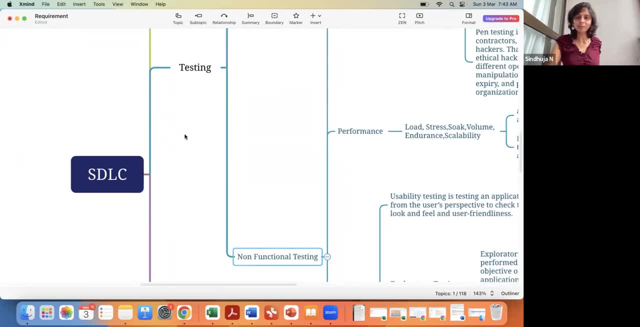 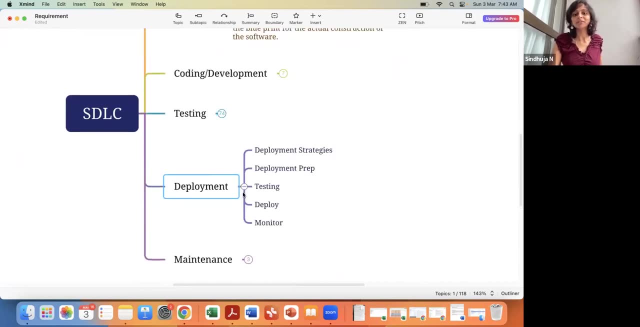 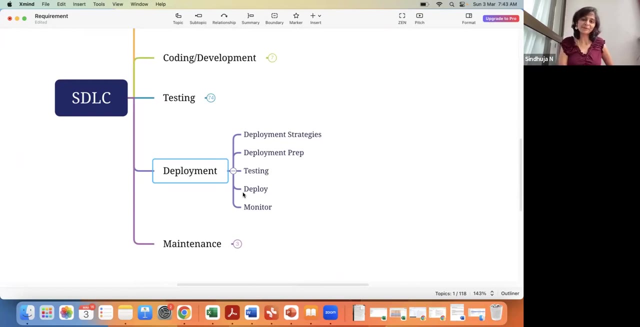 these kind of testings will happen. take will happen in the testing environment. okay, and deployment: deployment is something crucial. early days deployment is something, if i, if i remember correctly, still uh, during the testing environment, and the testing environment will be used for the testing environment the weekends only. the deployment happens before deployment. we want to prepare a big strategy. 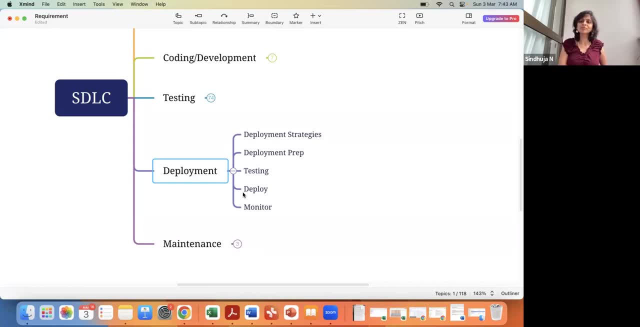 documents and environment, set proper version controlling and the weekend we should be in office to make this deployment happens and some operations teams will be there to do and help us with the deployment. okay, but nowadays in agile razor, working in the cicd pipelines devops, the concept of development plus operations comes together. these things are getting better. 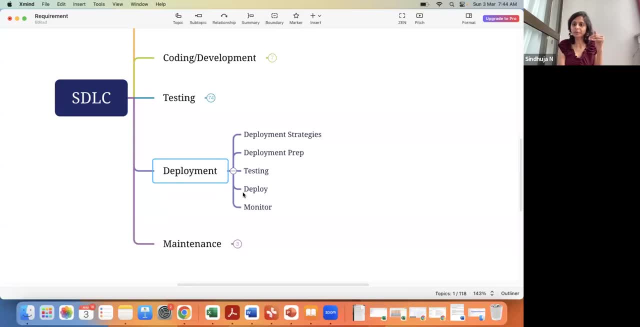 and easier for us to do so. the deployment strategy should be there. how are we going to deploy? at what point of deployment? the strategies should be in place before we do department deployment, preparatory activities, testing, deploy, monitor. okay, so this is how it is so. once after, uh, we 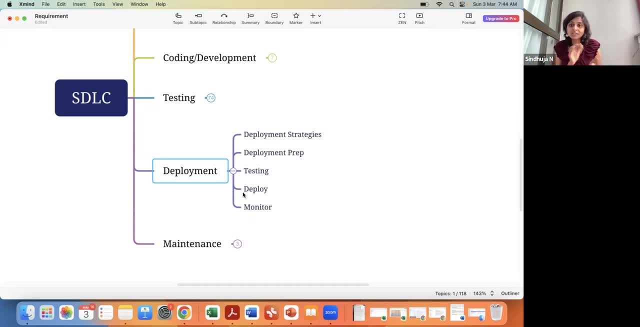 move the code, these, the developers, will do some kind of basic testing and then they will deploy after deployment also the production environment. we will just do some sanity checking whether this function is some basic important functionalities are working properly like that. we will do check monitor, then only we will return home in early days. 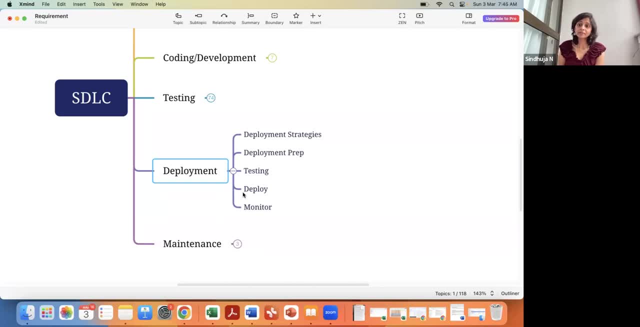 nowadays everything is becoming automated. deployment happens, even in amazon and all. if you see 0.68 milliseconds, they will say like that deployment is happening quite, quite often. so there is no schedule and all. deployment is very frequent in the retail industries and and maintenance. so once after it deployed, of course we may have on top of it some enhancements, some bugs may be there. 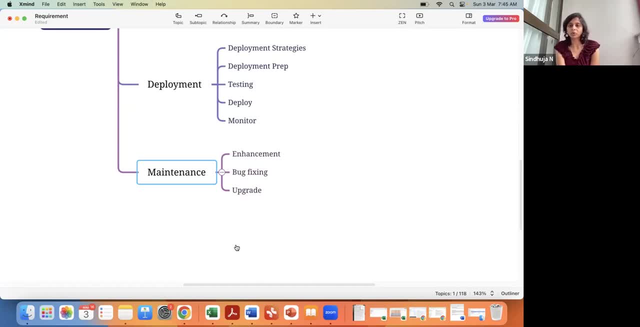 okay. it's quite common and quite acceptable. whatever we are doing, it cannot be perfect all the time, and there is no such a term called perfect as well. so bug fixing, upgrade, enhancements when we want to do this, maybe when we implement the system- i have been into those upgrade projects and all. 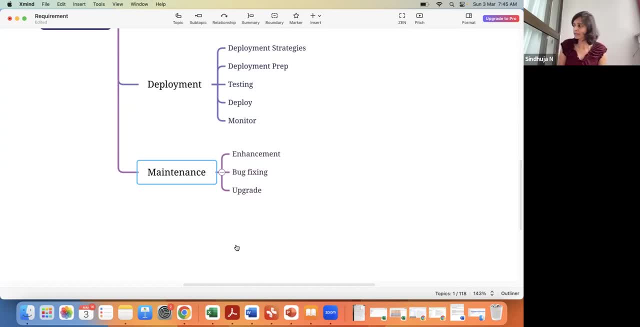 we must have been using some way back software. so tools, that kind of things should be replaced now. so that kind of upgrades things will happen in the maintenance. okay, so in maintenance we can do enhancement, bug fixing, upgrade in a gel ways of working. this can be that baikanban it's up to again. 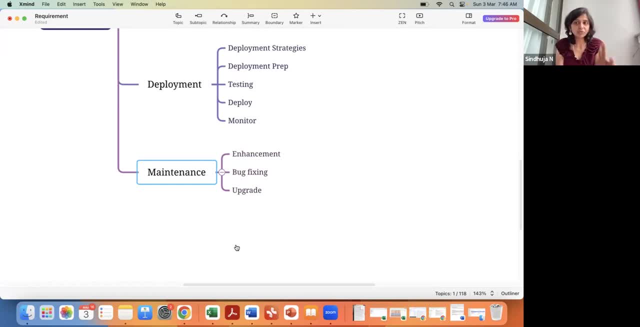 organization team. they can decide, if suppose this kind of activities are coming, which framework is best for them. enhancement, if they might go for scrum or something else, or even they get could get up in kanban itself. it depends on the scope, it depends on the organization and they think how they.